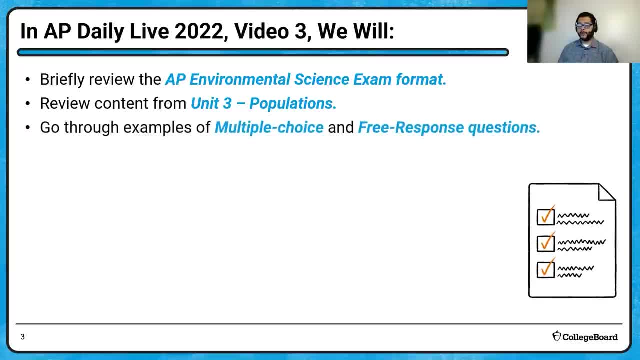 teachers And we will try to get to go through another couple of examples of multiple choice and free response questions, So that way we get some practice There And of course we will be reviewing the science practices and the skills that are most. 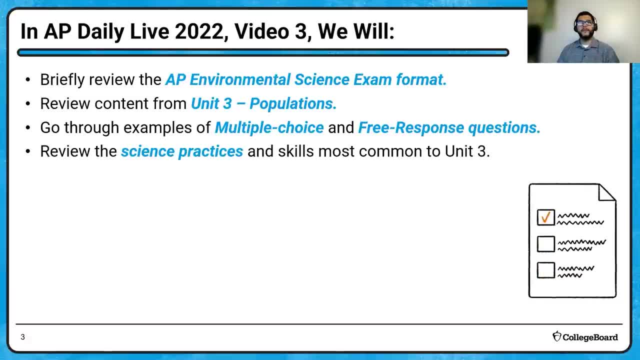 common for these, for this unit- Because that's an important thing- is to make sure that you're prepared for what's likely going to be on the test, And of course, we'll also recommend some AP daily videos for some more in depth practice. And then, at the end, after we've gone over all, 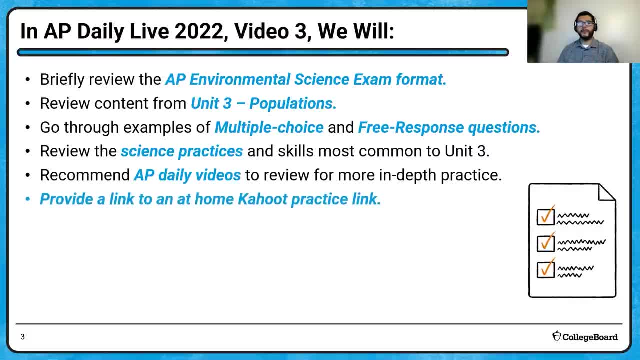 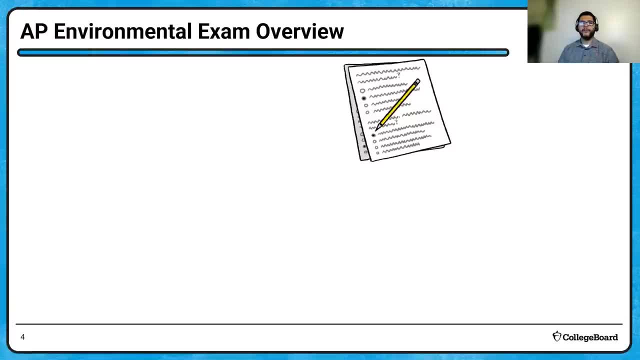 this. we will be providing a Kahoot link for you to have some practice with some of this material. Okay, All right, so let's get going. So the first thing is remember we do have two sections to our exam: multiple choice with 80. 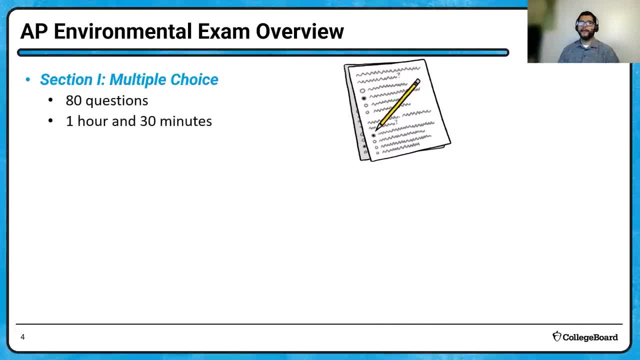 questions. that will be an hour and 30 minutes And that does involve 60% of your exam score And we went through in the first video. please make sure if you want to go review those. the different multiple choice questions: there are standalone questions And there are sets with 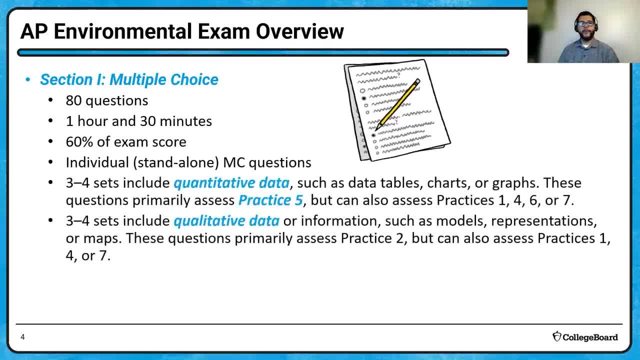 quantitative and qualitative data assessing all the practices all the way through 71234567, which we'll look at in a minute, And there will be also some text based questions that are only assessed through the multiple choice. So if you have more questions on those, please make sure to review video one, That one. 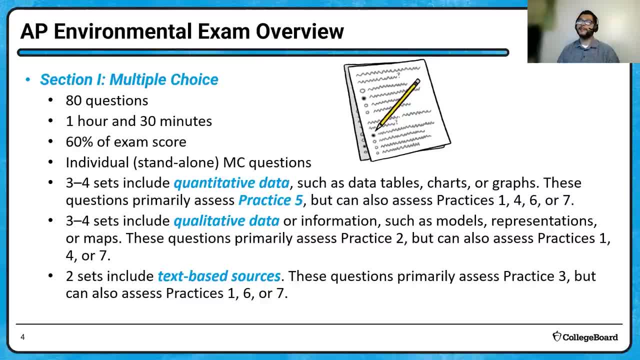 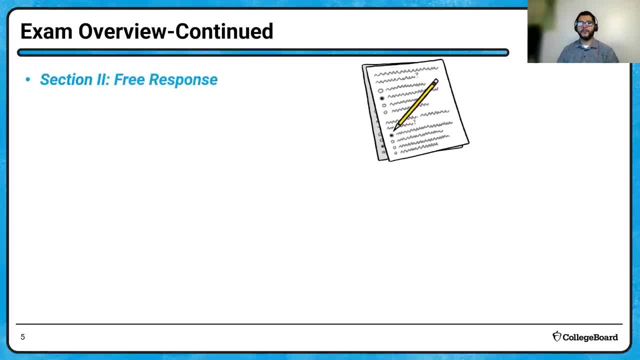 does have a good in depth. look at all the different questions, plus lots of examples, So please make sure to check that. And then, of course, FRQs will be a part of our test or free response questions. There are three of them, which gives you about an hour and 10 minutes total And, with some reading, 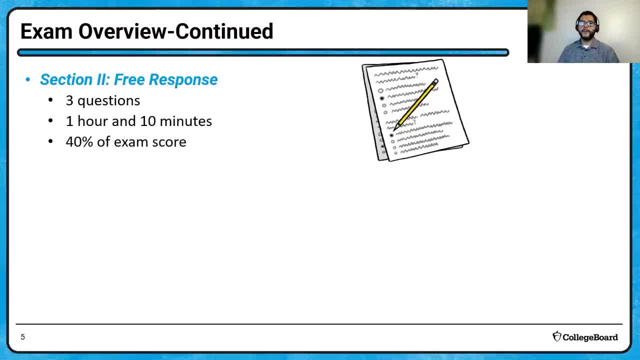 time. that's about 20 minutes per questions And that gives you 40% of your exam score. And the formats are always the same. So question one will ask you to design an investigation And it'll ask you questions about other investigations And then 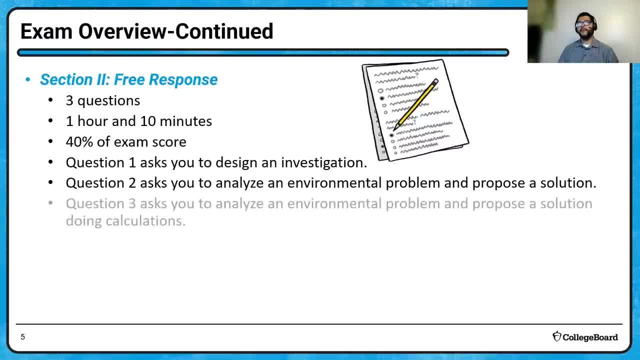 you'll have to analyze a problem, proposed solutions And then, of course, you will also do the same- analyze and propose, but doing calculations as well, And we'll talk a little bit about that today. we'll talk about multiple choice calculations and see how those are included as well. 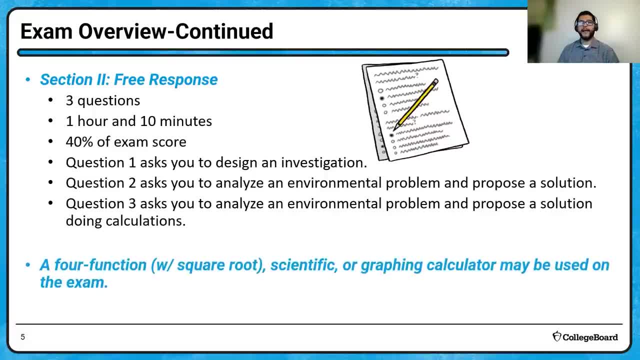 And then our four function calculator is allowed for this either scientific graphic calculator as well, And that's a good thing. So hopefully that'll help you guys out. All right, and this some helpful links. If you'd like to pause the. 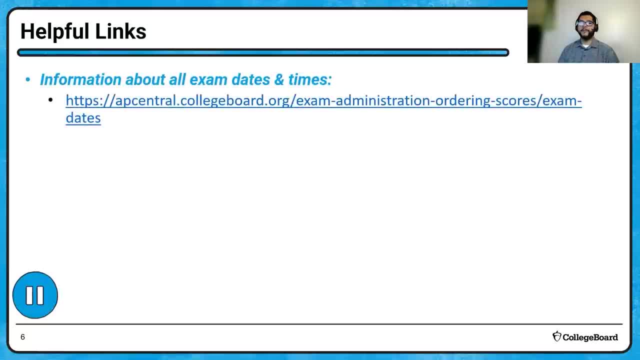 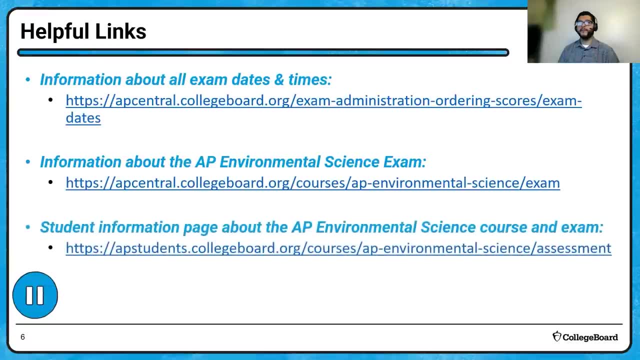 video after you see these. these are going to be about the exam dates and times for all the AP classes and courses. This is going to be about, specifically, the Environmental Science exam And then for student information on the course and the exam and some extra study materials. 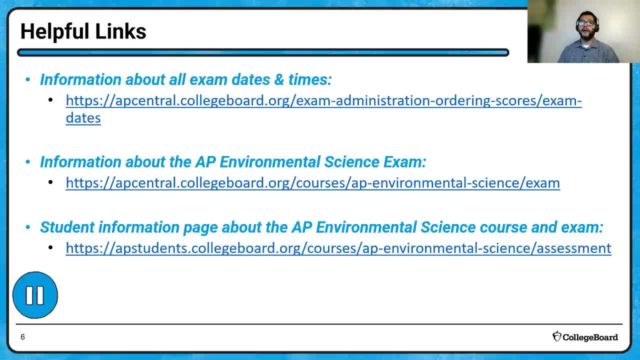 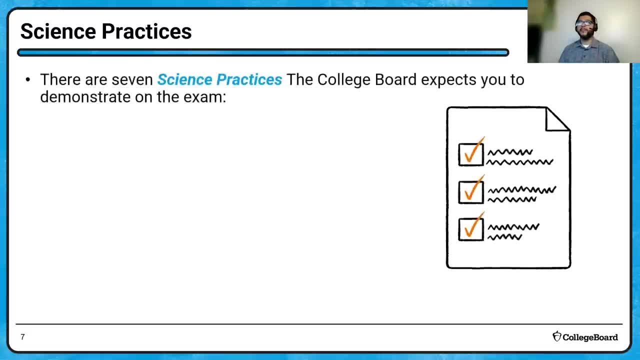 as well. So if you want to pause that and or take a picture of the screen there, that would be helpful. Okay, and then the science practices. So remember, there are seven of them, And the College Board is going to ask you questions that are going to have you demonstrate those skills. 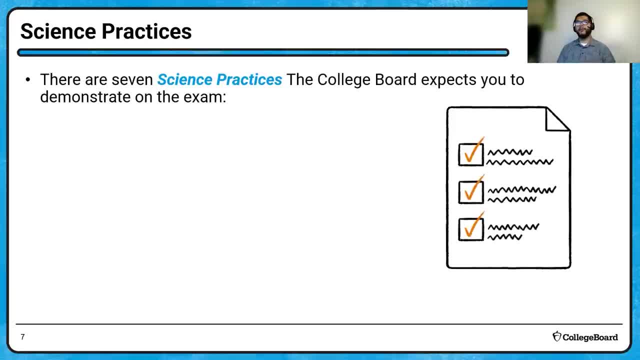 on the test. So for sure you'll be seeing them in the multiple choice and the free response. So concept explanation is going to be the main one. where do you know this info? there'll be some with visuals where you'll have to look at a graph or a chart and or maybe a diagram of some. 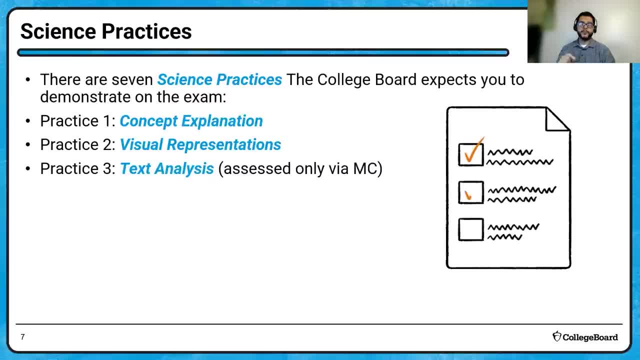 sort right. And then text analysis is only a multiple choice, So please review that from video one. And then, of course, today we're going to be looking at scientific experiments. That's practice number four. And then we have data analysis, where you're looking at graphs and 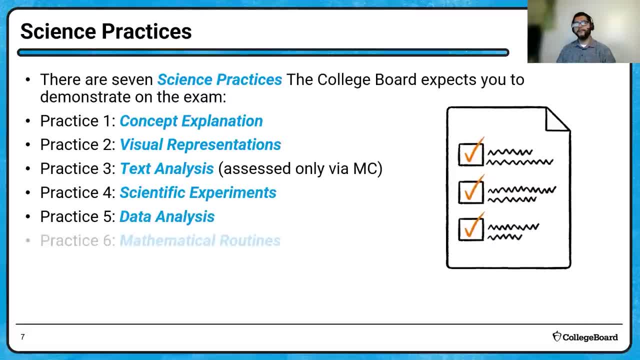 charts and either made to predict or make conclusions on those. And then, of course, we have the math routines, which are going to be a part of today's video as well, because we're in unit three And that's populations, which is a very, very good section to talk about math. And then, of 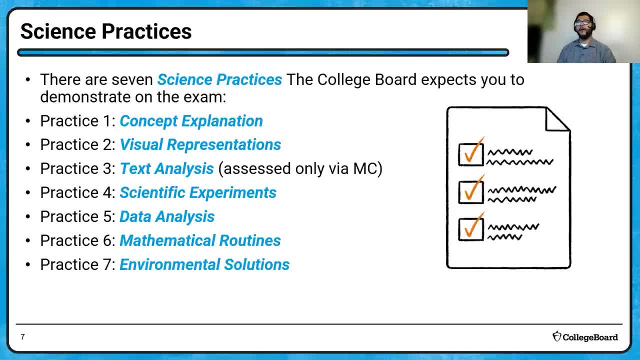 course we have environmental solutions. So while we are going to focus on certain skills and practices on this unit and we have in previous units, we need to make sure that we understand that they can be assessed in any unit for pretty much any practice. Okay, All right, So let's go. 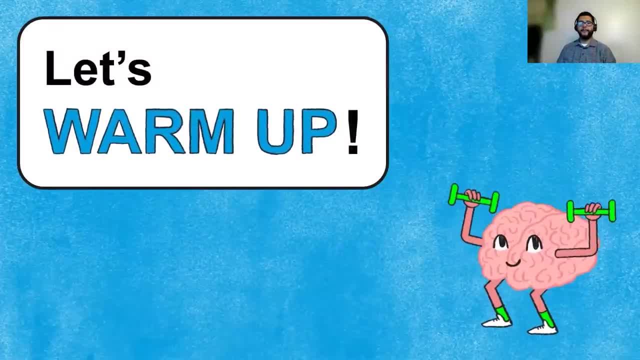 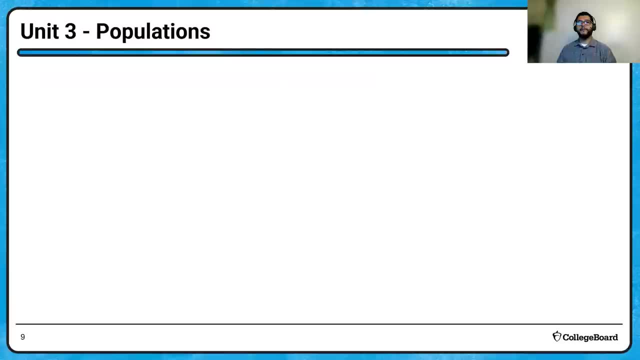 ahead and warm up with some review from unit three. Okay, So Now again, we won't be able to go over every everything, but let's try to do as much as we can and try to get you as much information as possible. So some of the content from unit three: 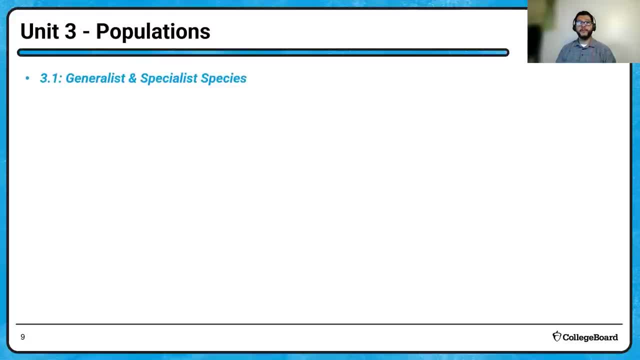 Remember, we started off with generalist and specialist species And this is going to bring a big vocabulary word that we always talk about in environmental science and that's the ecological niche, that's the role that an organism tends to play in their environment. so we're talking about 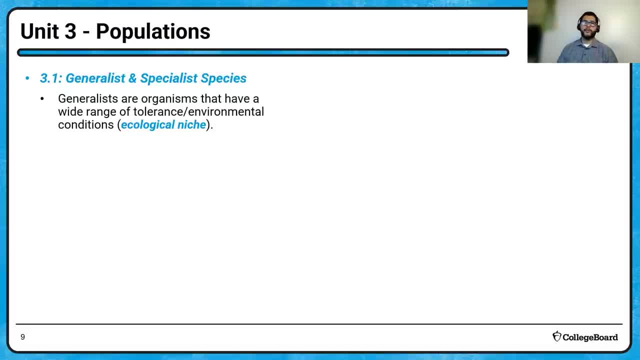 whether they're appropriate or not, Okay, producer or a predator, or on the third trophic level or the second trophic level, or whether they're an invasive species or an introduced species. that's going to be part of our ecological niche. And, of course, range of tolerance is something we talked about a little bit previously. 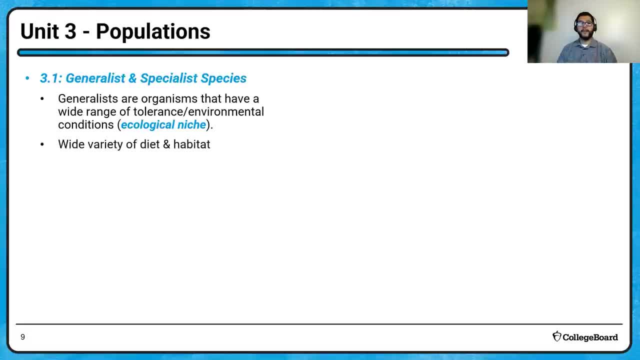 as well. So please make sure you know those. And so those that have a wide variety of diet and habitats, those are going to be your generalists, like raccoons, bobcats, coyotes, And they tend to be the kind that, when introduced somewhere, they can become an invasive species. And then 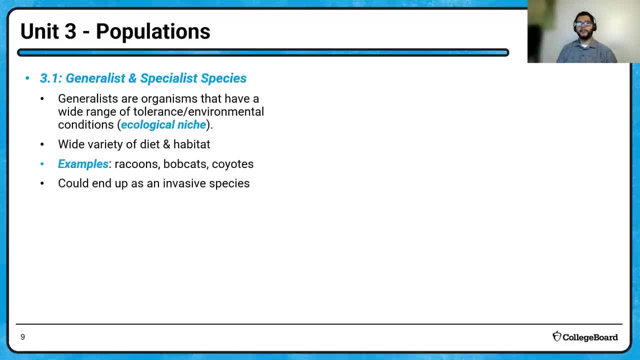 when we have our specialists, they're going to be the ones that have a very narrow range of environmental niche, And so they are going to have special things that they have to eat. So, for example, those are going to be specialized diets, habitats that are required for them to survive. 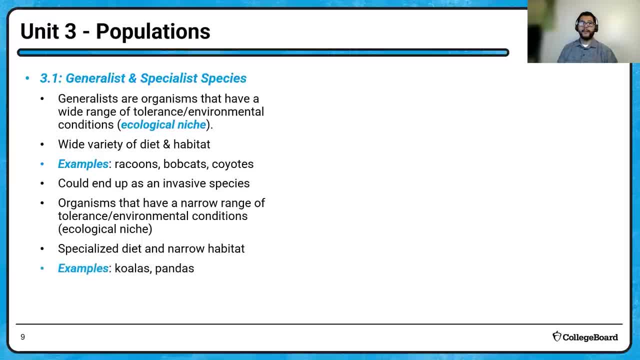 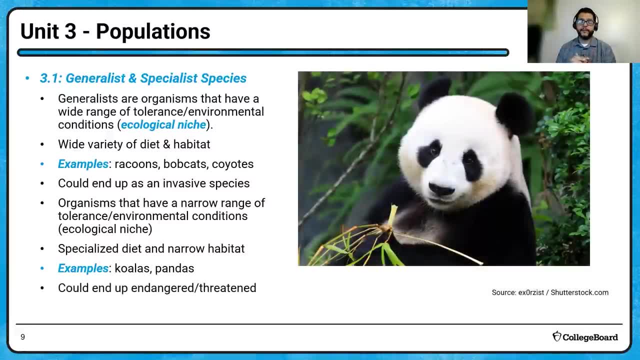 So good examples of these are koalas and pandas, And they could end up endangered or threatened. So, you know, when you see a panda, they're a really good example. they have a specific type of bamboo that they like to eat. They're very picky when it comes to, you know, choosing a mate And because 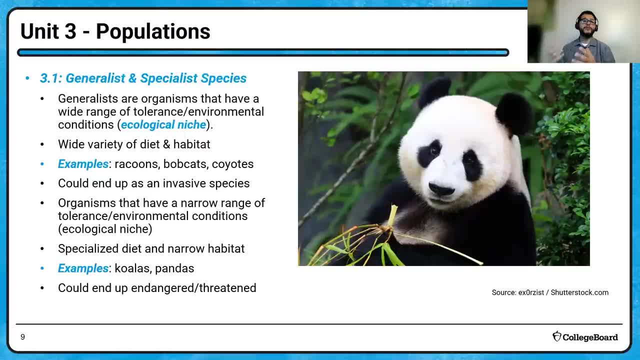 of that. they're an endangered species And they're kind of end up being the poster child for for endangered species and specialist species as well. And then, of course, if you know anything about koalas, you know they were devastated by wildfires in the last couple of years as well. 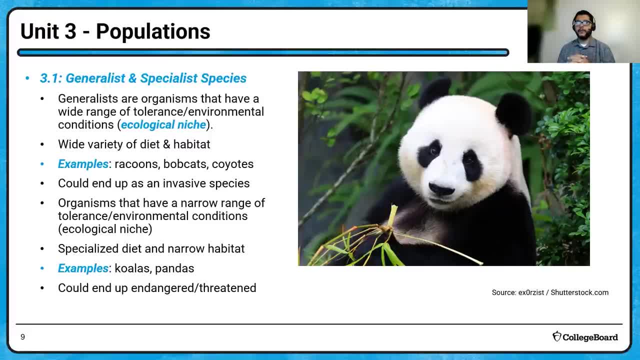 So that's because they're certain species And then they're pretty much the actual predators of certain eucalyptus leaves. So that is very different from a raccoon, which will quite literally eat trash, And so that's something that we tend to joke about in my class. So if you hear the phrase, I'm sure you've heard of the phrase. 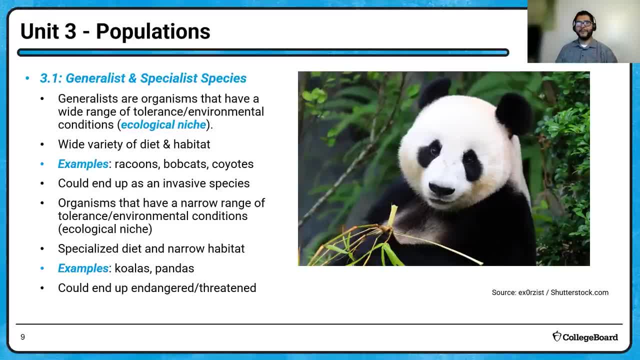 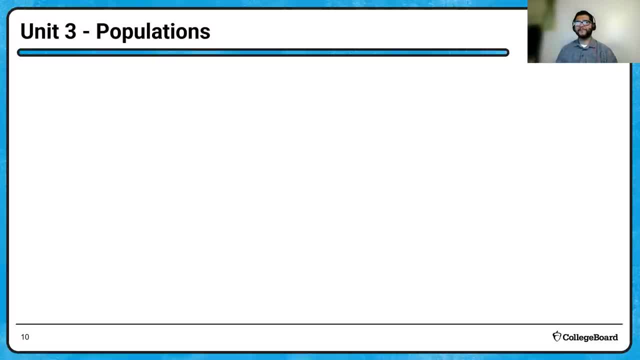 trash panda, and that's a raccoon. So definitely something you would like to do if you're living with humans, but not if you're going to be a specialist. So Okay Now, moving on on. Now, this leads us into how these species are able to actually reproduce, right? So some? 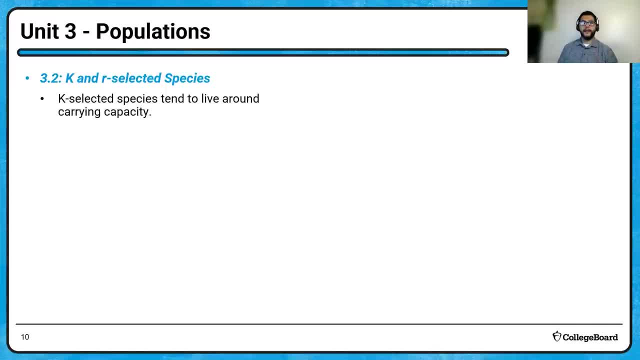 species like the K selected, they tend to live around the carrying capacity right. So here in this section make sure you understand the differences between K and R selected. So K is all about carrying capacity, R species: they like to live around that reproductive potential, So in 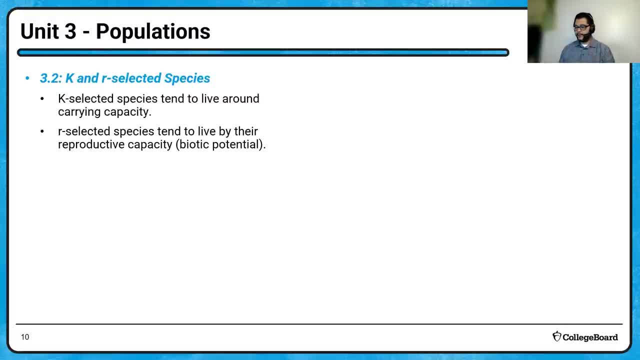 other words, if you're thinking about a J curve, right, If you're thinking about your typical J curve, they tend to go for that all the time. So when we're looking at it, let me go ahead and show you my drawings here. So if we're looking at our curves here, then that J curve, that's kind. 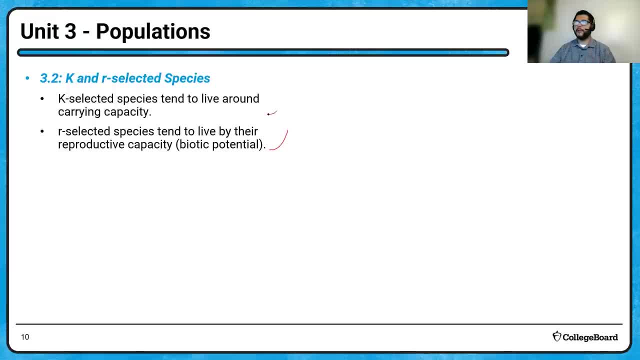 of where they live, whereas, opposed to the K selected, they're more along the lines of up- excuse me, they're more the lines of up and then flattening out right, Not all the time, but that's pretty close, And so not all the species do end up. 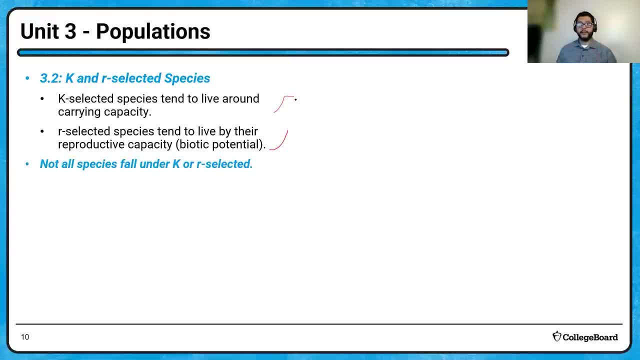 falling under the K or R selected right. Some have different conditions and may have to change strategies. And then K selecteds can be affected by those invasives pretty often, So that ends up being kind of an issue. And then R selected species. they tend to become those invasive. 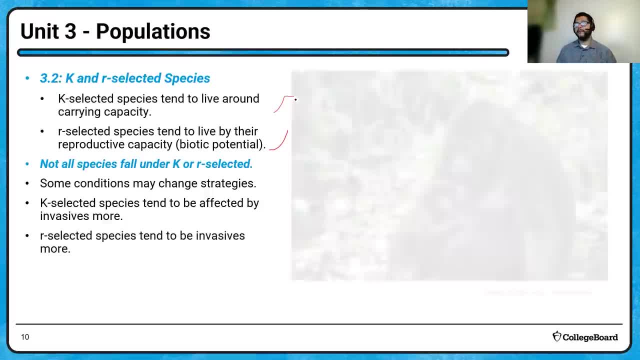 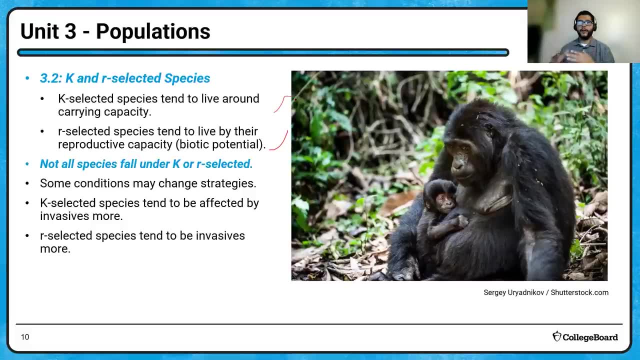 species. So that's going to be an issue we have there right, And so mammals tend to be large. mammals tend to be these K selected species because they have certain criteria that they can't be affected by, And so they tend to be affected by those invasive species. 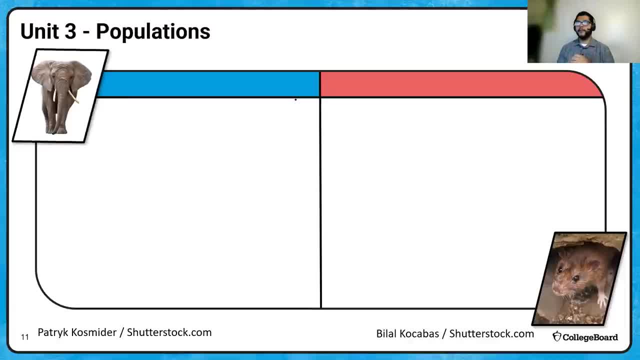 They tend to meet. So if we take a look over here, here's our examples. right, The, here's two mammals, but one of them is more K selected, One of them is more R. So if you look at the elephants right, Elephants are very large species. They're K selected. They tend to have 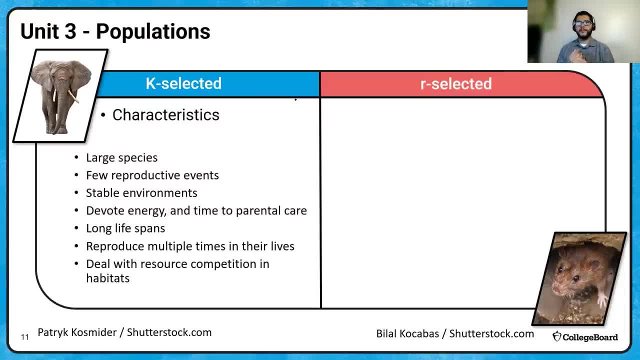 few reproductive events. Some elephant species can be pregnant for more than a year or two years, almost, right. They tend to live in pretty stable environments and their energy is basically for parental care, right, And they tend to have very long lifespans due to this. And then they do have. 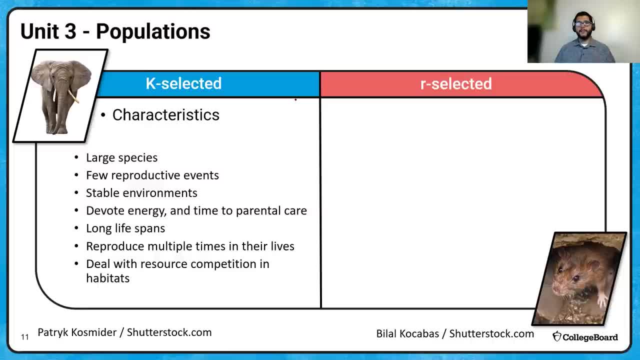 multiple reproductive events, So they are not limited to just one reproductive event and that's it. So that's something that's very different from an R selected. And then of course, they do have to deal with competition for those habitats. Now, an R selected species, they tend to be pretty much the 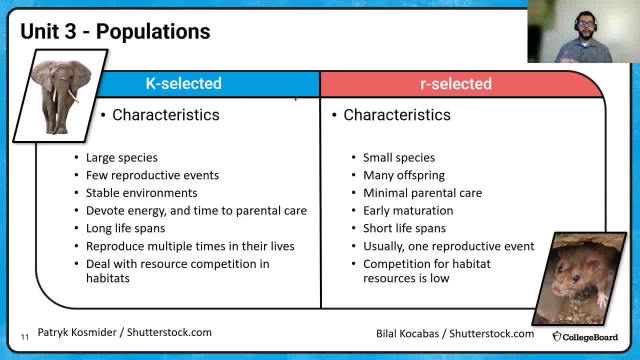 opposite. They're smaller. They can have many offspring in one reproductive event. You know, think about salmon spawns, Right, Salmon go up river, they spawn like crazy and then they die afterwards. So that's tends to be something along the lines of an R selected. And then, of course, you have minimal care for parental. 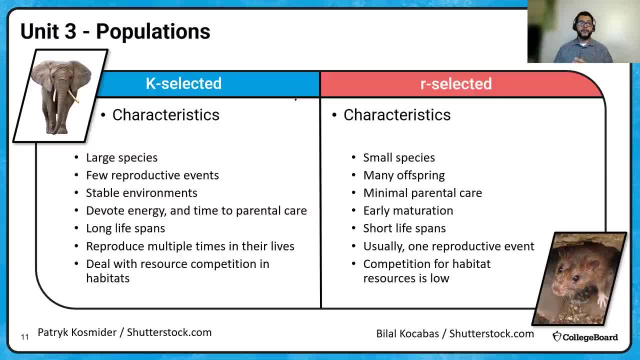 for those species And of course they mature pretty early. So that tends to be a characteristic of them is that they're ready to breed and then move on Right, And then of course, their competition tends to be low, because they're not- they're- long enough to compete, Whereas like 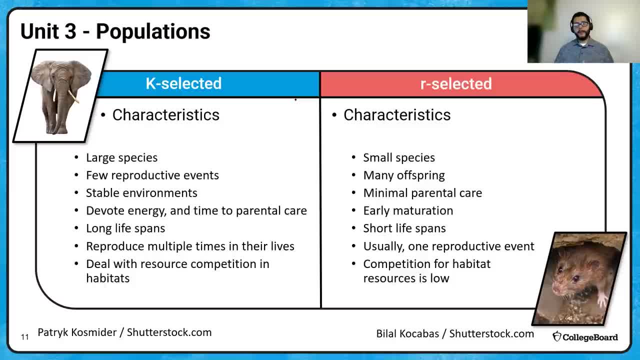 if they're an elephant, they have to travel, they have to make sure they have water. They may have to make sure they can find food, and you know, for mice or bugs or fish or salmon, that's not a concern of theirs, It's just a matter of okay. well, let's live as long as we can to breed, Right. 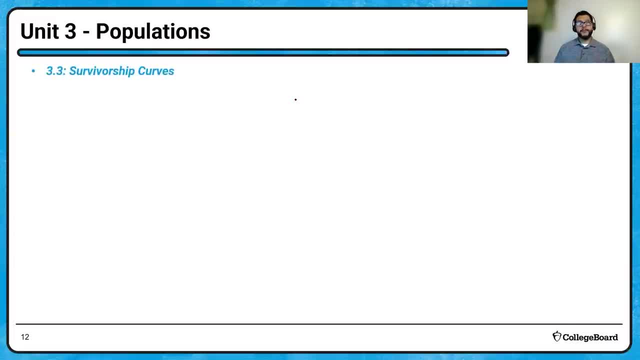 So from there, this leads us to survivorship curve. So one thing you're going to notice about unit three is it's full of graphs, Right? Of course I mentioned the S curve and the J curve, That's, your logistic growth and your exponential growth. But another one that tends to confuse students a little bit is a survivorship curve. Okay, So you have to be pretty aware that this is a line that's going to show how long a species can survive, Right? 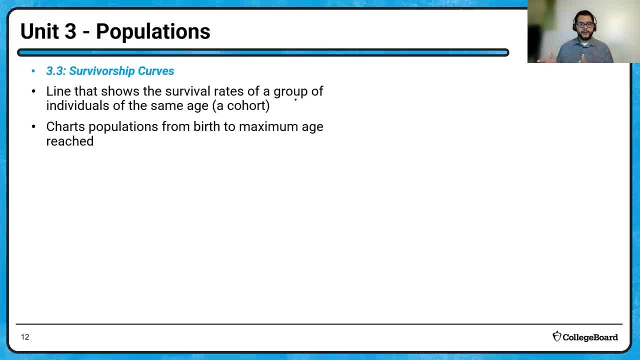 And again, this is not how long in a number of years set, it's how long for that individual species. So, basically, from birth to their age, how long are there? And so we have three groups, right, We have type one, type two and type three. 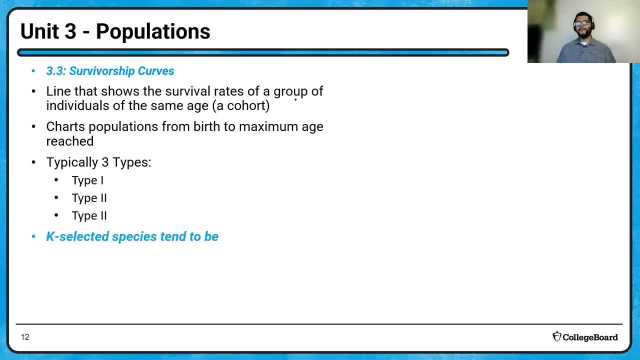 Okay, And then K selected. they tend to be that type one and type two. Okay, They show up and they are either long lasting or they end up being at a constant loss, but it's not a massive die off, Right? Whereas in our selected species they have, they tend to have a lot of individuals at the beginning and then very few of them make it to old age for their species, Right. So if you take a look, okay. 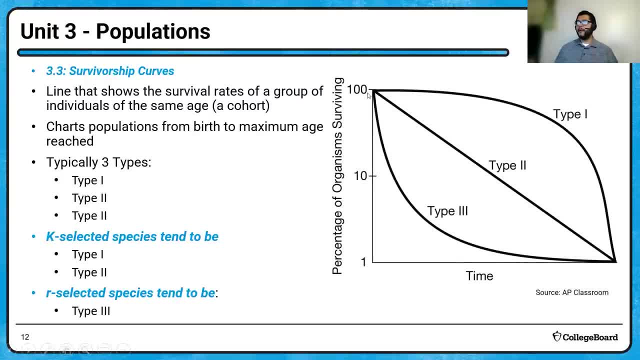 So here's our different types. We have type one where- and again, this is by time in their species, And so this is not how many years in specific numbers. So when you're looking at this type one, these tend to be your large mammals, right. Many of them survive their youth and then they don't die until they get older. Type two would be something more along the lines of a squirrel or a bird, where they are pretty much a chance of getting. 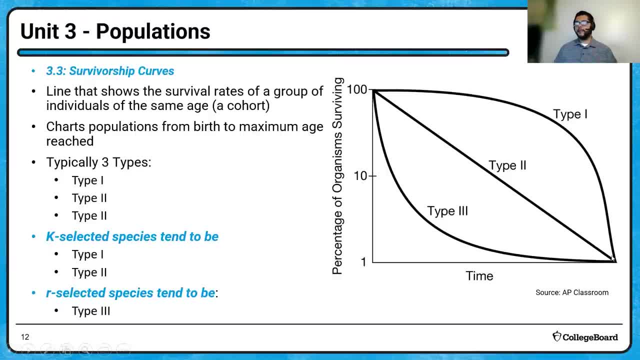 old, You know, lost at any age and then eventually everything goes back to zero, Whereas over here this would be like your mosquitoes or your salmon. they would have a very large number at the beginning and then a large number would die early and then very few make it to older age. So know that chart. it's going to be one that likely will show up, And if they don't actually show you the graph, they'll probably ask you a question about you know this species would probably fall under which type? So make sure to know those. 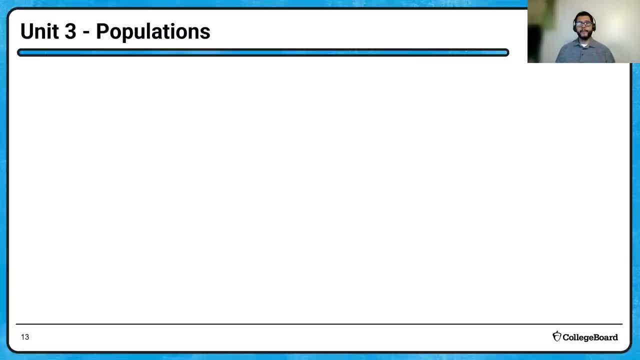 And that's very related to that, R and K selected Okay. And so we mentioned carrying capacity and those logistic and exponential curves. So be familiar with those right. Carrying capacity is going to be, how big is the population going to be before it runs out of food or shelter or requirements? And again, here's something that I want to make sure that's clear, because students tend to get confused about it, is that there's not a definite line. 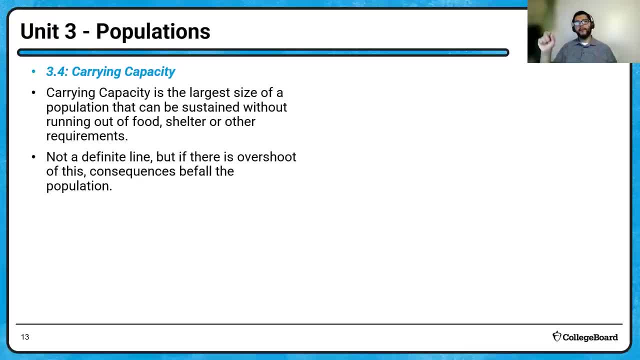 So we end up going over a lot And then we end up going back. So we call this overshoot right, And that's going to be where we go beyond carrying capacity. because here's how it goes, guys. Species don't get a memo saying, oh hey, we've reached carrying capacity. no more breeding until no, that's not how it goes. A population will continue doing what it does. 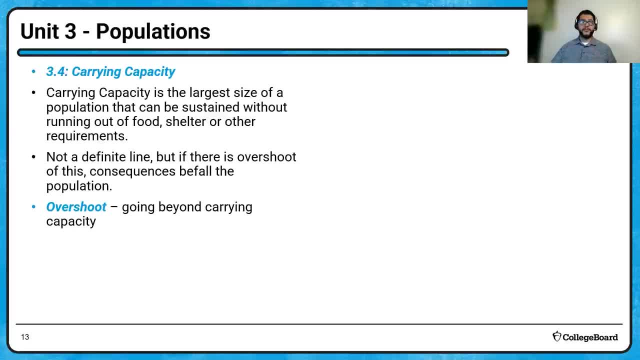 And you know, for most species, that is to pass your genetics on to the next generation. So breeding becomes a goal of biological populations. And then, of course, you have resource depletion being a common consequence, And once that happens, then you get dieback. Okay, That's going to be where the numbers drop because resources go down. So that may be a famine disease or, in the case of a human population, conflict right. 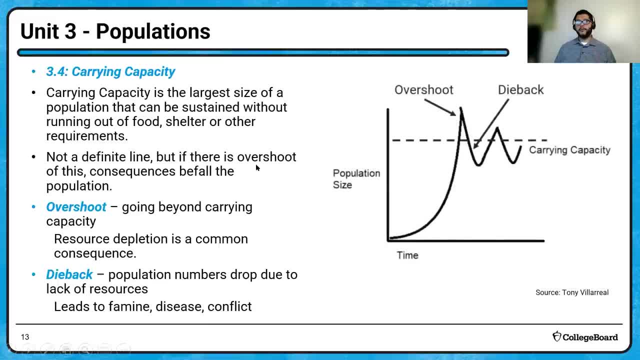 So quick side note here, just to kind of pause for a second here is to make sure we understand when I talk about populations or when anybody talks about populations, I like to put these into two groups. We put them into biological populations. 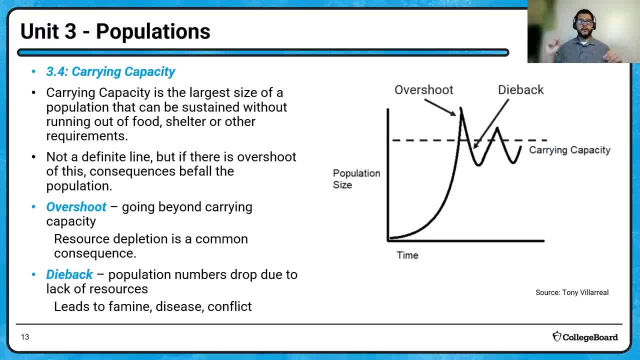 And then human populations. So when we're talking about carrying capacity, overshoot, dieback, these apply to both groups, but there are certain things that only you're going to hear about humans. So when we say conflict, that's probably a more human characteristic or human population. 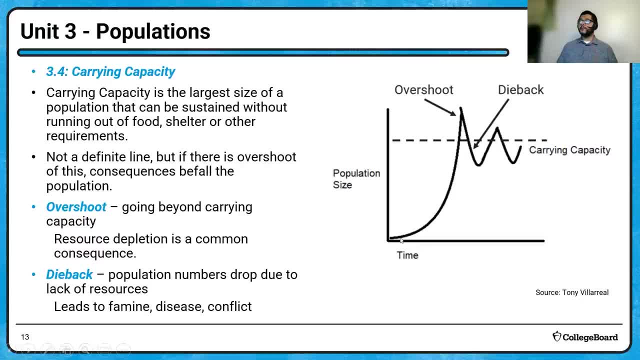 Okay, so just keep that in mind. And then you look right here, here's our typical graph. So you see, there can be overshoot where the numbers go way up for a while, and they're right there. If we section this off and we look at it right, this is our J curve right here, from here to there. Okay, that's your J curve, that's your exponential growth, And then most populations don't go to carrying capacity and then just level off. That's not the case for the most part. 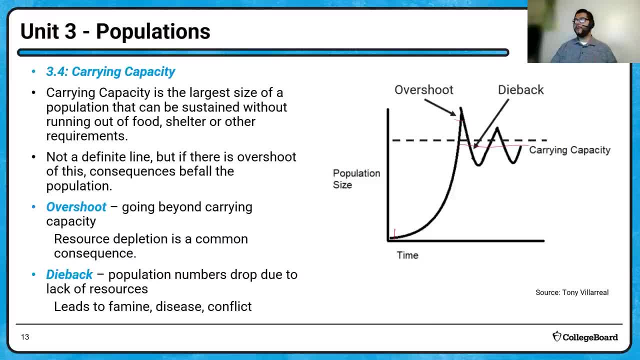 What happens is you end up with an overshoot and then a drop, and then a smaller overshoot and then a drop, and then that continues until it eventually kind of evens out Around there, Okay, so just be aware of that. That tends to be the case. 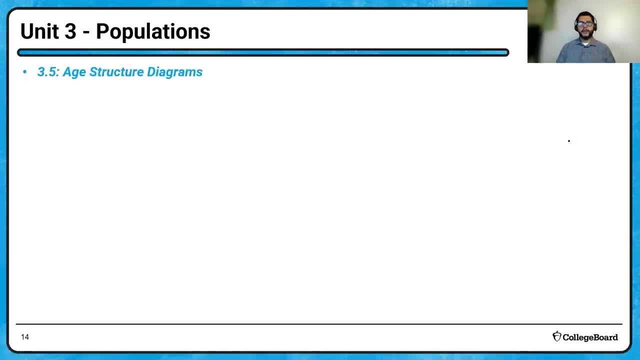 Okay, And then, of course, this leads us to a little bit more human populations. So now we're looking at age structure diagrams. You probably know them, and I always call them a population pyramid, Right? And this shows the distribution of the ages in a group, as well as the sexes in a population, so you can see where they are and how many there are. So when you look at the shape of the pyramid, it tells a lot, right? 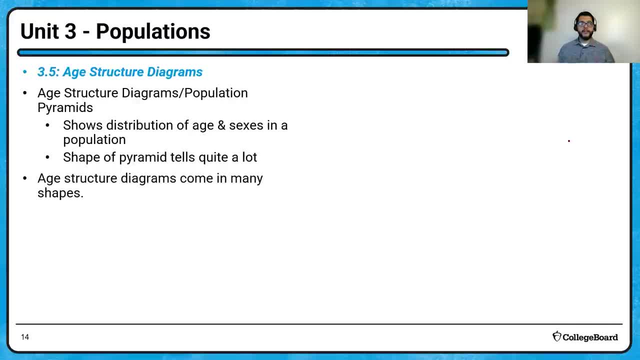 Okay, And so these diagrams can come in many shapes and, of course, they can tell us the trends. So if you see a population pyramid that is bottom heavy, that population is going to be growing, and we'll talk about it in a second, once I show the graph here. 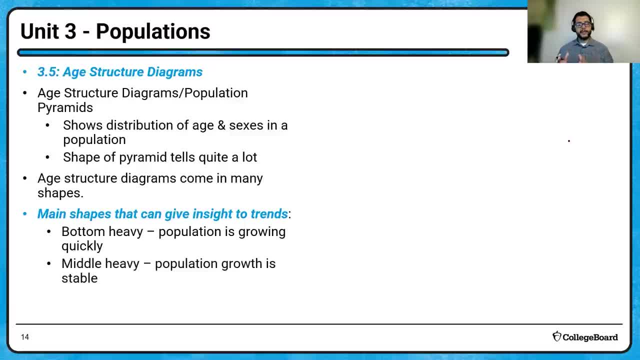 If it's heavy in the middle, that population is going to be pretty stable. it's not going to be at a point where it's getting too big and it's getting to a point where it's over growing right or growing too fast, And then we have ones that are 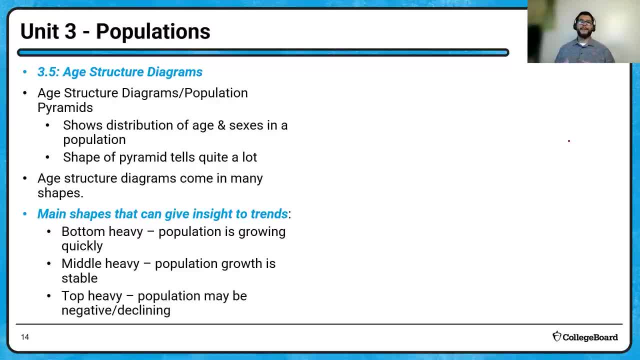 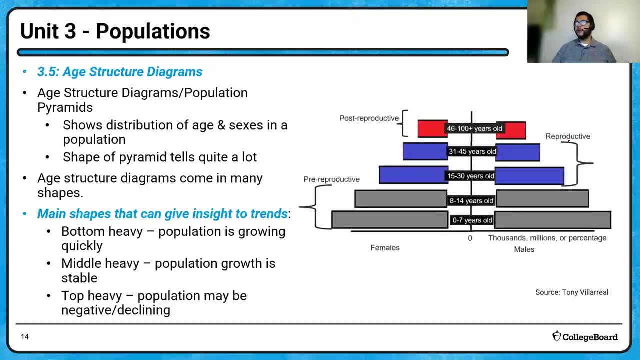 Population pyramids. that can be top heavy and that's going to be where it's in: a declining or a negative population growth. So let's take a look at what they look like. Okay, So here you have your typical groups. we've got pre reproductive. that's going to be those that are considered too young to meet. 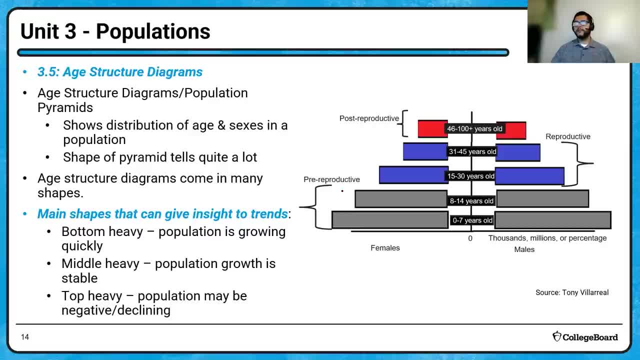 And have children. So you know, between the ages of zero to 14, the population could be that pre reproductive, whereas a population in the reproductive stages is going to be anywhere between 15 and around 45. And I do want to make a note of that. 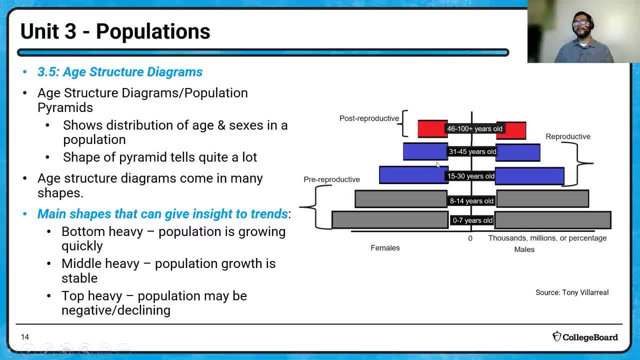 And I do want to make a note of that, And I do want to make a note that when we talk about this, about this, these groups, we tend to mean female groups, because they're the ones that continue to have babies until about that age, and then they stop. 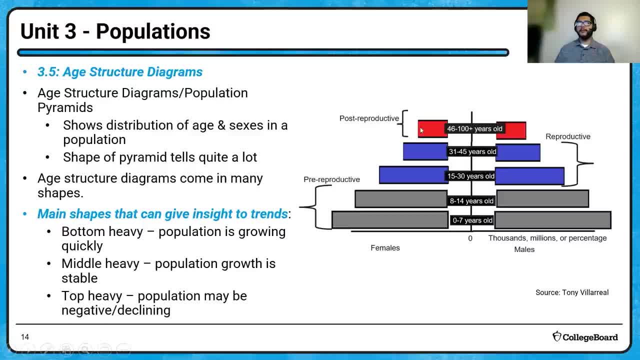 Males can continue, of course, into the post reproductive ages, but typically that's not a driver of population growth. And then over here you can see in this shape right here this pyramid is bottom heavy. So we'd probably say that this population is growing. 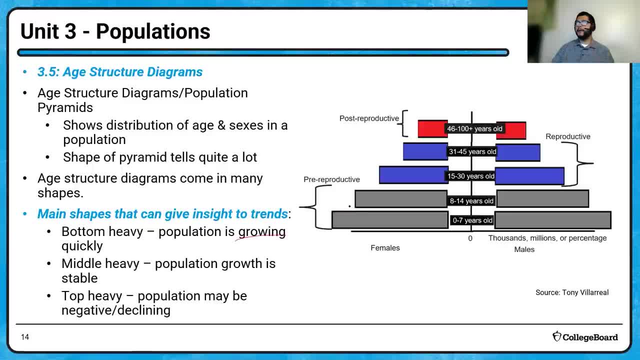 Okay, And so that's an important key, And so that's an important key there, And so if this were wider in the blue sections then it would be a stable, and if this were wider in the red sections then that would be more of a declining population. so make sure that we know what those trends are. there's almost always a picture of these graphs or a description of it, and then you have to answer questions on that, both in the multiple choice and the response. so make sure to be aware of those. 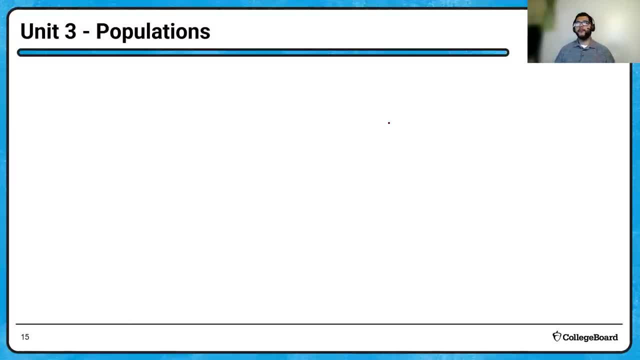 Okay, And then for our populations- infertility rate and human populations- that tends to be an important factor that we want to look at right. So, if we look at total fertility rate, This is something that's a difficult concept to grasp, but something that's super important. 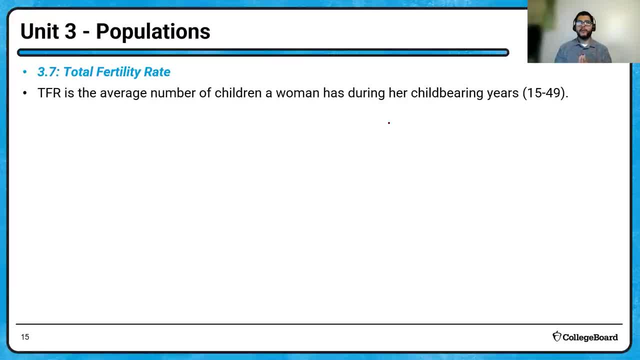 The idea is that we can look at the average number of children a woman is going to have in those childbearing years, typically from 15 to 45 or 49. And that's going to show an average rate Of babies that can have. and, of course, you're going to see numbers that are decimals. 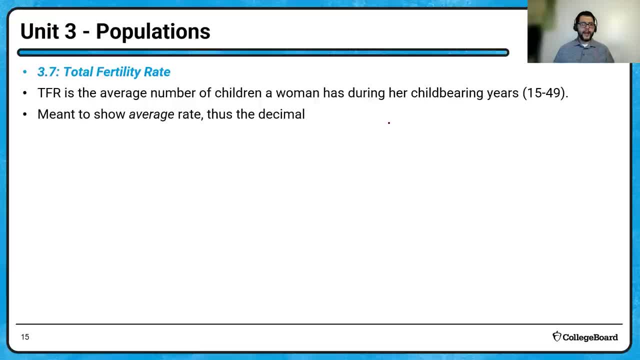 You know, it's not that you can have point six, five of a child, It's that it's an average. so that's where you get the decimal Right. So currently our world total fertility rate is about 2.5.. Now this differs depending on whether we consider the country a developed or developing nation, Right? 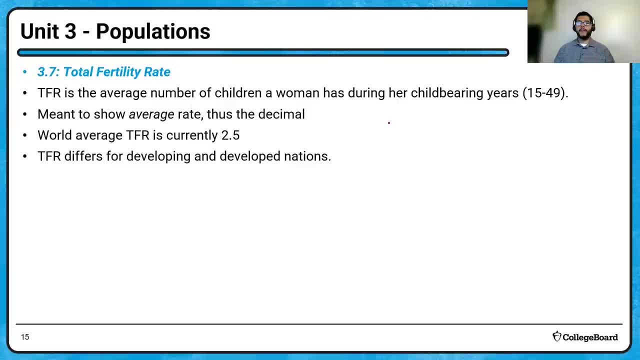 And so those developing nations. They tend to be those that have total fertility rates. They tend to have total fertility rates above 2.1. Some countries in, possibly, the African continent. They tend to have population or total fertility rates of six or seven right, so that's an average lifespan. a woman in those countries tends to have around six or seven children. 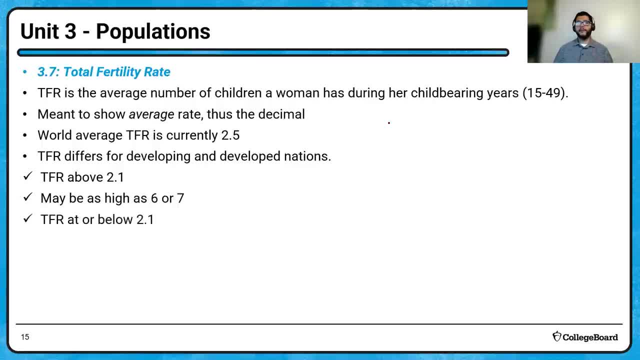 Whereas in a developed nation they tend to have a total fertility rate below 2.1.. Okay, And so that fertility leads to much slower growth and that's going to lead to the population having kind of a bigger chance of decline. Right, And one thing I do want to make clear is when we look at the factors on what is going to affect fertility rate, 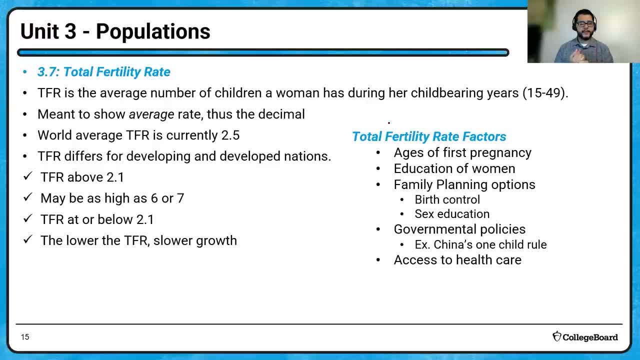 The biggest ones are right here. so, first of all, it's: when is the first pregnancy? is it early on? because, if you think about This, is a country that's considered developed Right. You guys who are practicing to take AP exams likely are not planning on having children right away. you know, you plan on going to college because you're taking a course. it's going to give you college credit. 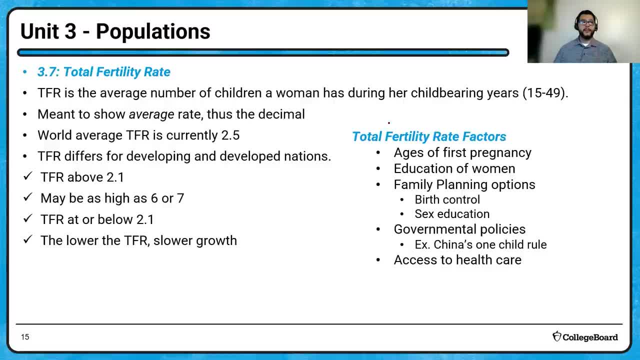 And once that happens, you're probably, you know, not having children very, at a very young age. Statistics will show that And that's going to be an important thing. so if that young, If a woman is not that young when she has her first child, then that's going to really bring down that fertility rate, because that is less time to have children. and education is probably the most important one, and specifically of women, because the more 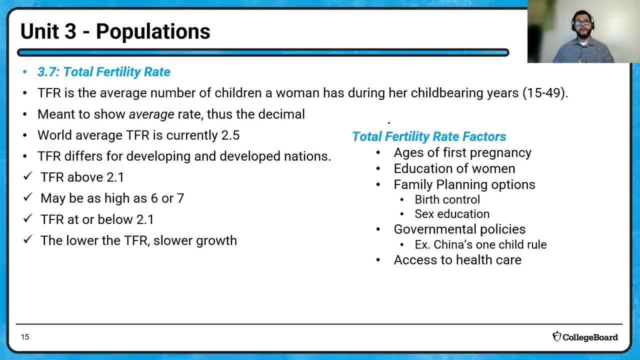 women are educated, And the longer they are educated then the less chance they will be spending time having children. And of course there are other factors. So this is where we kind of blur the line between our course and maybe a government or an economics. 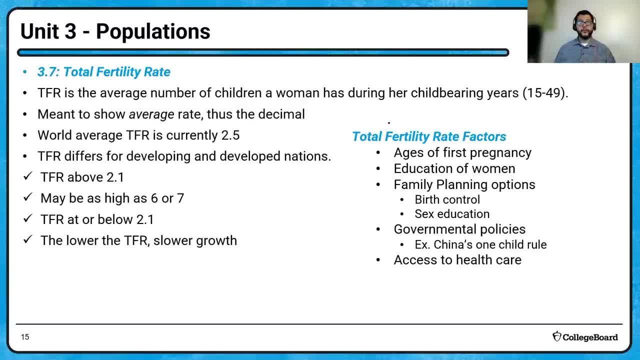 course. There are family planning options. you can have birth control, sex education. There are governmental policies that can be enacted right. China had a one child rule for years and it wasn't anything you know. it wasn't anything other than you would get taxed for having more children. 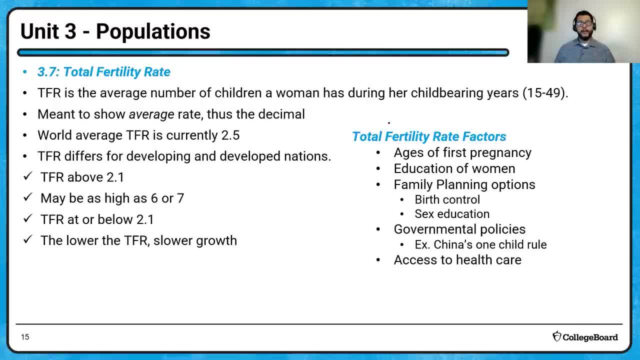 And if you had female children, the taxes would be higher. Right, And of course, access to health care. so if those, if those factors change, that's going to have a very, very significant impact on the total fertility rate. Right, And of course, I would say, probably if you have to ask, if they ask you a question where you have to say what's one of the most important ones. 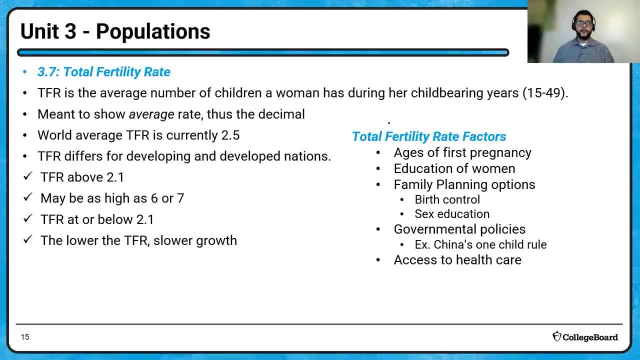 Education of women is probably the biggest one, because the fact that women choose to be educator have the right to be educated. in some of these developed nations That reduces the amount of time they're going to spend having children, so total fertility rate will go down because of that. 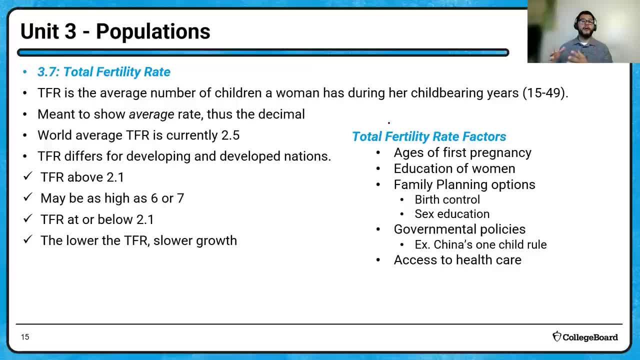 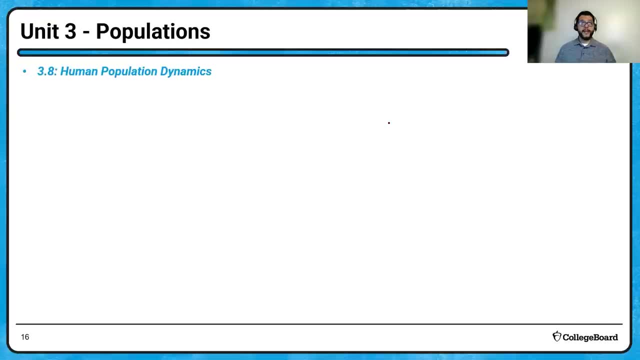 And again, remember, this is something we talked about with human populations. We're not talking about this, We're talking about this in biological populations, because this is a very different thing when now we're talking economics and social sciences as well. And, of course, when we get to the human population dynamics, there are things to think about. right, just like a biological population, there are factors that affect us. right? we have birth rates, death rates. 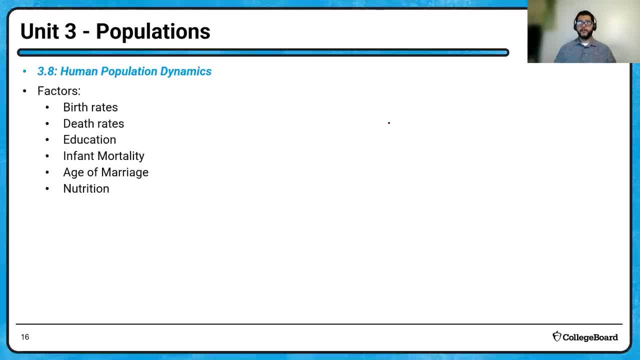 But then we get to things that are more social science, right education, infant mortality, the age of marriage and, of course, nutrition. that's a big one too, And so you know, back There was a economist who was named Thomas Malthus, and he had this idea that all populations have a carrying capacity, even human populations, and that at some point the human population would likely end up being in a very dire strait. it would end up having a problem. 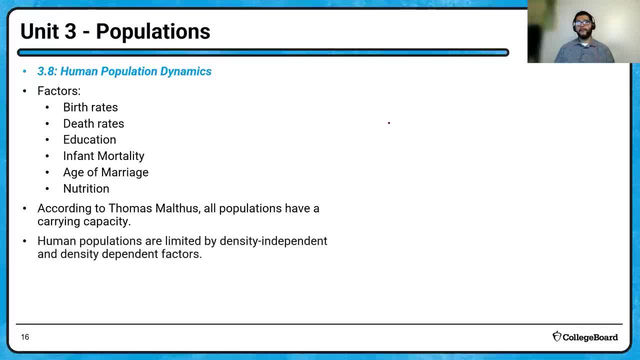 with food production And that we'd have maybe density independent And that we'd have maybe density independent And that we'd have maybe density independent or density dependent factors. right, And we're going to go over some of those factors in the next video when we talk about food production and land use, because, because of certain strategies which will be to be continued tomorrow, 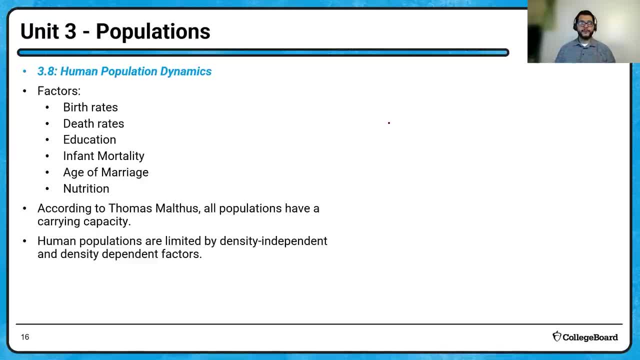 We've avoided the, you know, kind of gloom and doom that Thomas Malthus proposed right, And so some of those factors we do have to consider are those that are density dependent. so that means that the more individuals there are, 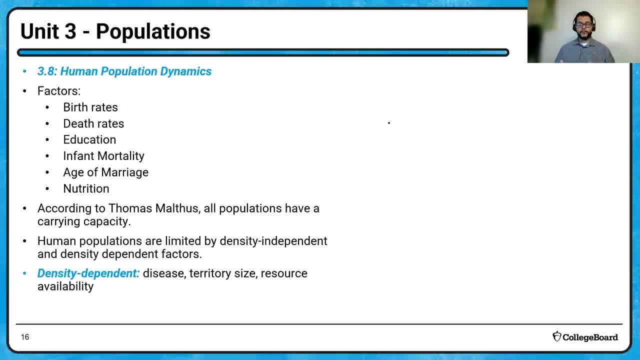 And so some of those factors we do have to consider are those that are density dependent. so that means that the more individuals there are, Now some of these factors, whether we're operating on food or if we're operating on the environment, 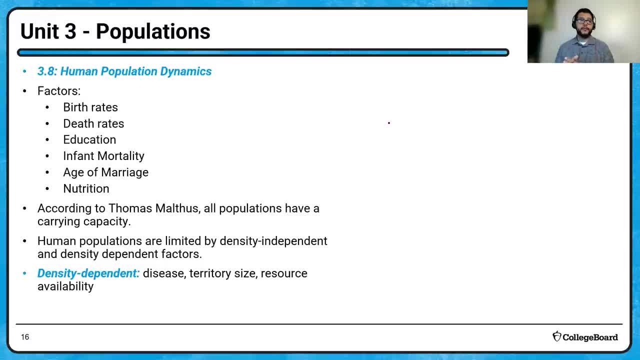 We're operating on the environment itself. We're operating on the environment itself. make sure that you're, you know, able to hold on to your nest while you go out and still find food and things like that. So that's a density dependent. Then of course, you get density. 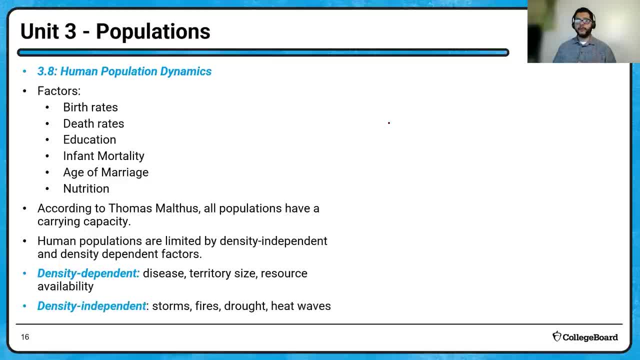 independent. That would be like storms, fire, drought or heat waves. So in the cases of human population density, dependent are going to be relying on, think about urban cities right. Or disease or famine. Those are going to be issues where the more of us there are, the bigger those. 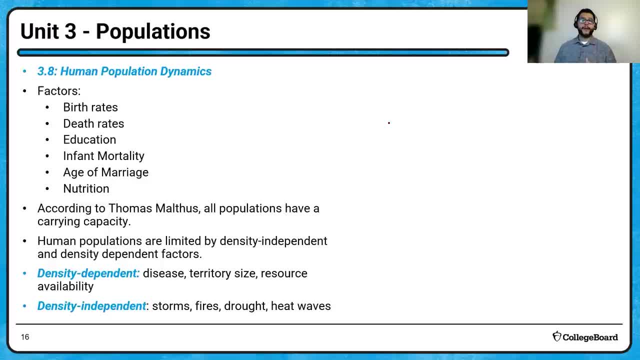 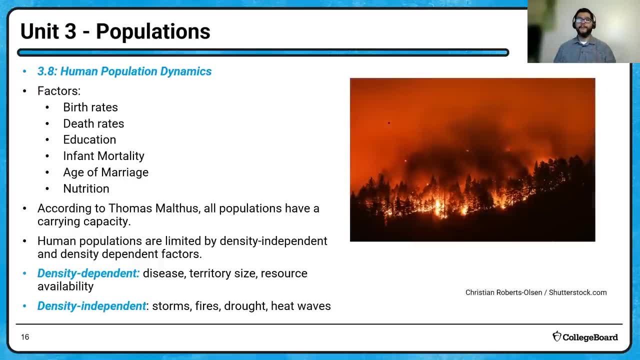 problems are Density independent is going to be something like a tornado or a hurricane. The population will be affected by those you know in the event happening, no matter what. So if you've got you know, 10,000 people living in the path of a storm, or if you've got you know 200 people, 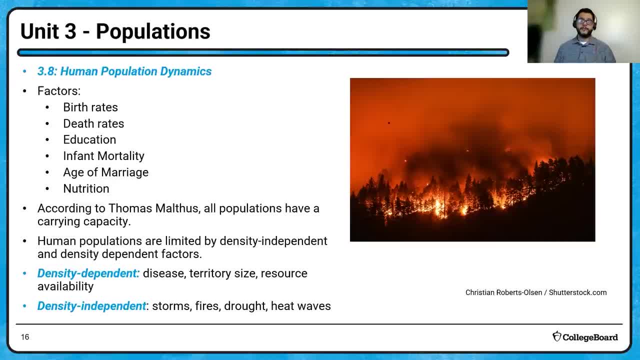 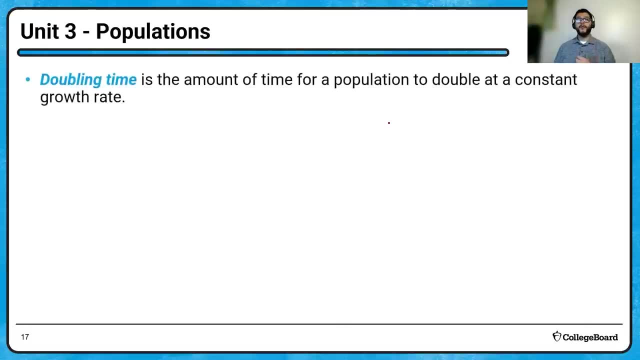 living in the path of a storm. it might have an impact on populations. So, luckily, we as humans have, you know, been able to get around some of those issues with forecasts and things like that, but it is still. It's still something that we have to think about. Okay, And now we get to the portion where we talk. 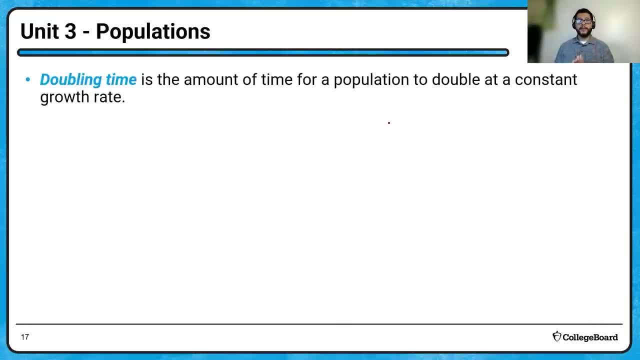 about the math. Okay, So doubling time is an important thing. So a reminder: we do not get a formula chart for the environmental science exam. So this is one of those equations where you're just going to have to memorize, And I know that's not something we want to hear. but 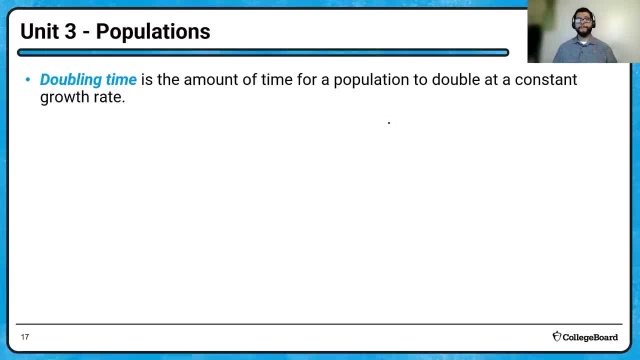 it is something that we do need to have. Okay, Now, doubling time is a big, big issue, because we tend to give you growth rates and percentages and then they tell you to calculate, And so this is the actual equation: It's 70 divided by R, where R is the growth rate. Now, this is a rule of 70. 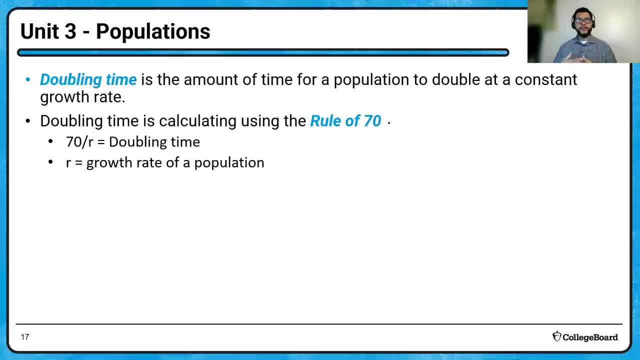 And what I will tell you is: I always get the question: Mr V, Mr V, where do they get the rule of 70?? And my clear answer for that is always: because math right. Actually, technically, it's because of statistics. It's a statistical number which you don't need to think about. So you actually have a little bit more incentive if that's where you measure the growth. but you don't have to think about any of those. You just get some control over the numbers. So an example of a number that was determined that we were going to be able to get ething out or get it to be able to get: 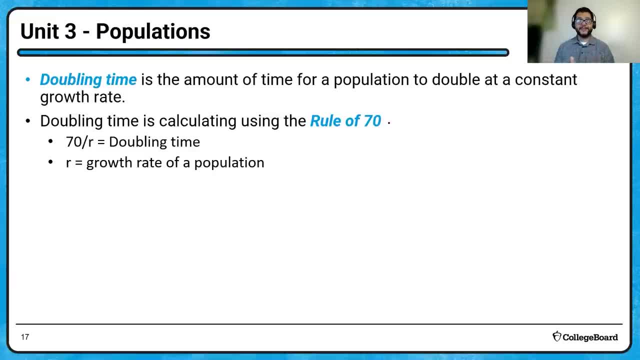 which you don't need to know the history of for our test. so that's a good thing, but it is something that we do need to have memorized. so, and if you ask a statistician, there are different rules for doubling time. there's a rule of 70 and a rule of 71 point. 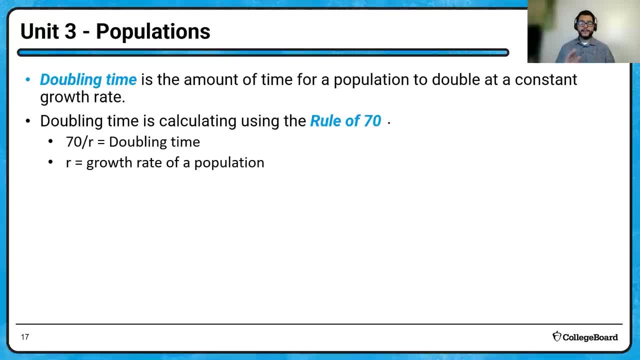 something and all these other things, but for us it's simple: rule of 70. okay. now what i will say about this is: they're going to give you, or you're going to calculate, growth rate and it's going to be a percentage. so let's say you're given the growth rate of 2.3. okay, what students tend to do. 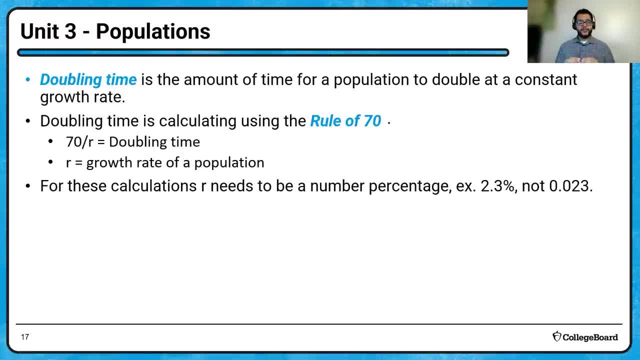 and something you should avoid is they like to change that 2.3 into a decimal and change it to 0.023, which is awesome, but that's not what we have to do. okay, so we keep it as the number percent they give us. so in this case, here's an example: if a country has a population of 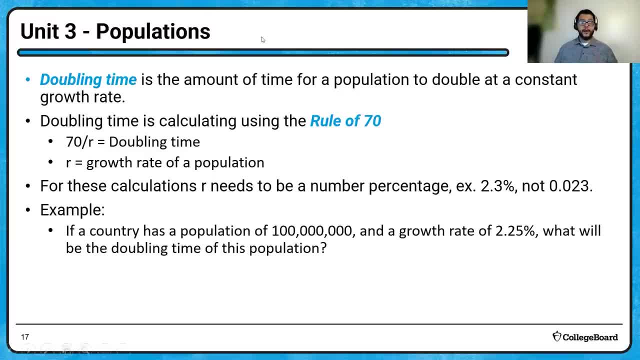 100 million and a growth rate of 2.25, what will be the doubling time of this population? so first thing i want to point out is notice the distractor here. okay, the number of the population here is a distractor. so this thing right here, we do not need it right, it's not important for this one. 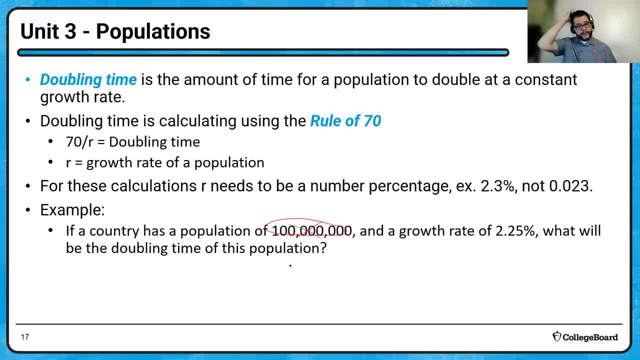 it's not asking us how much will the population be after a doubling time. it's asking us instead, what is the doubling time if they? now there will be questions where that does become an issue. so let's calculate the number of people who have a population of 200 million and a growth rate of 2.25. 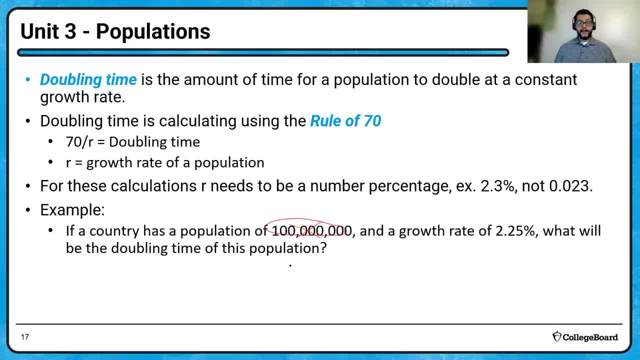 so let's calculate that. so we would take 70 divided by 2.25 and i get an answer of 3.11, 31.11 years, okay so, and again, this might be a multiple choice. if it's a free response question, sig figs tend to. 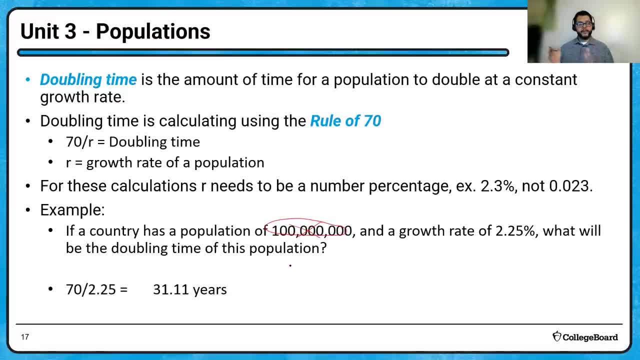 not be the case, as long as you fall within the range- and we saw that yesterday and we'll actually see some more of that, i believe, tomorrow in our math question and our- if our- cube. but as long as you're within the range of an answer, then you should be okay. right, and now a little. 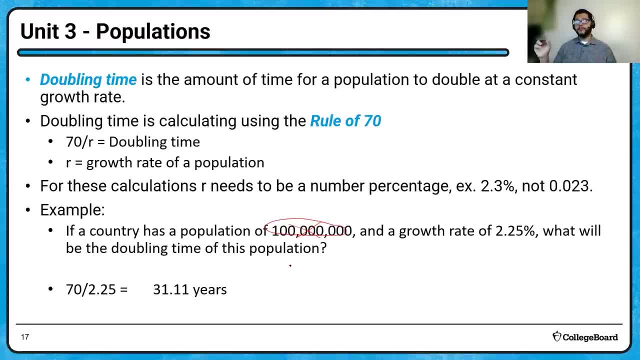 side note, if they do ask you to find the population, a second part to this question would be: what would the population be roughly in about 60 years? okay, if that were the case and it takes 31 years for it to double, that would be two doubling times. so that would take 100 million and double it. 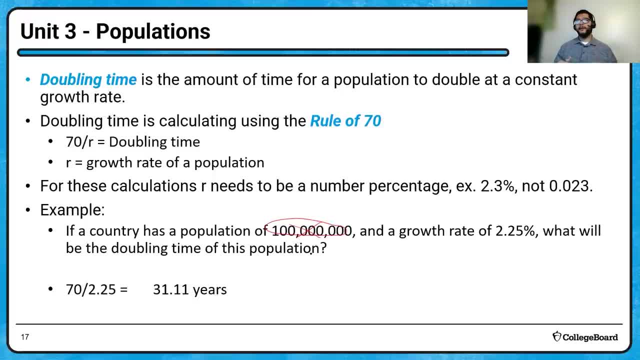 and then double it again, so it'd be 100 million and then 200 million, and then that 200 would become four. a lot of people like to just add the same amount each time, right, and they'll just go 100 plus 100 plus 100. that would be wrong, so just. 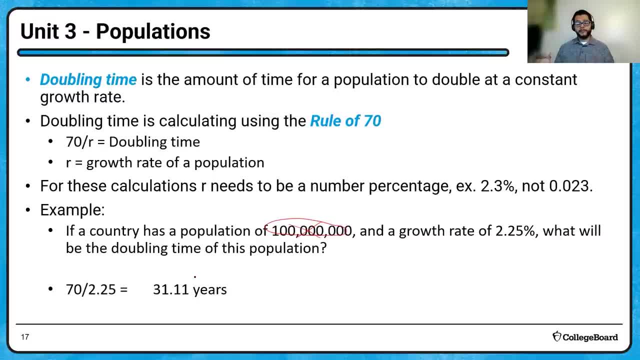 be aware of that. that is a question that may pop up, so look at that. read what's being asked you. that's a strategy we always want to talk about, so remember my strategies from the multiple choice sections: best to read and find out what you know and what you don't know and answer those that you. 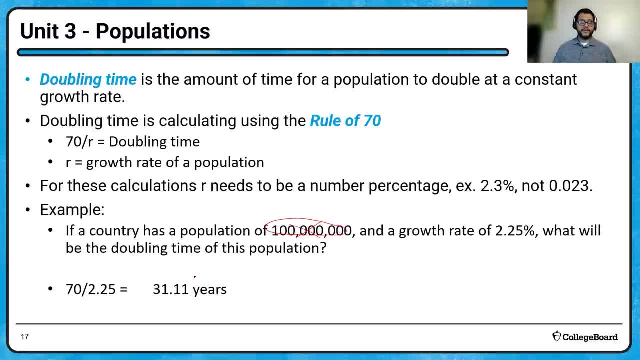 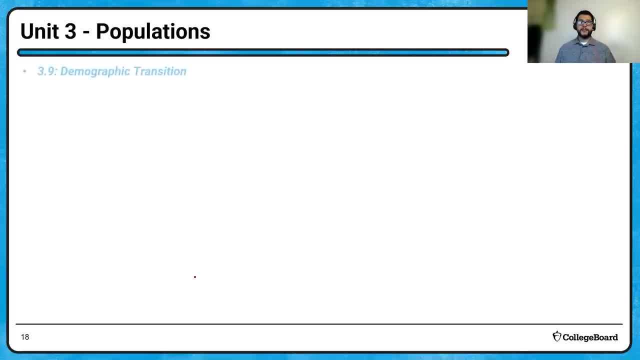 know first, and if this is an easy doubling time, then great, that's awesome. okay, then one of the last sections here for our populations is going to be demographic transition. so it's a historical model number one and it basically shows a nation and how they tend to go from uh population and birth and death rate. 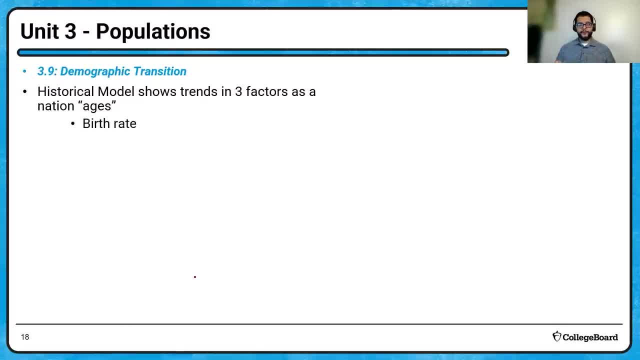 as they progress, right. so we look at birth, death and total population. okay. so we're looking at these three factors in one graph, okay, and nations tend historically to move towards industrialization. right, as we go from a farming or agrarian culture, we end up moving more towards industry, industry and that ends up leading our economics to change and our population. 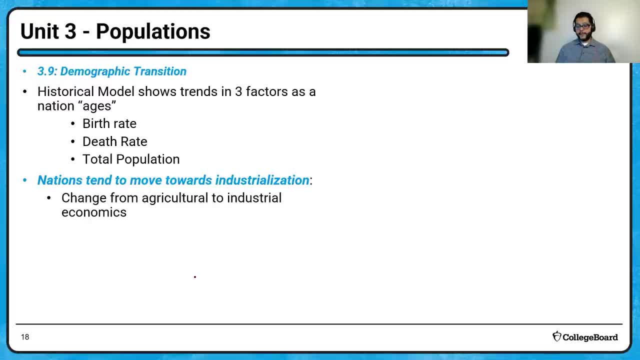 responds to this. okay, so we tend to see this typically through four stages. now, if you've taken ap- human geography, this also um is included. there's a fifth stage which we don't assess on the ap environmental exam. so we look at the first four stages and we have some kind of generalities there. so just be aware. 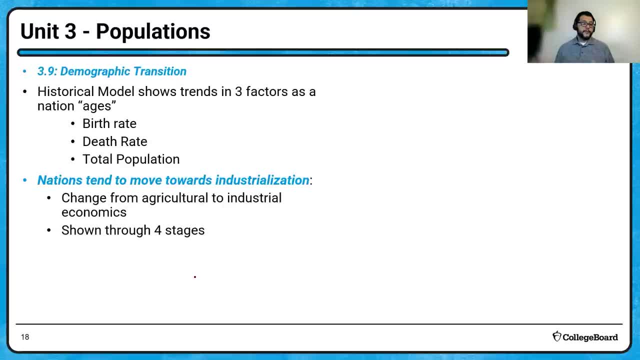 and i know some of you may have taken human geography and go, but wait. what about the fifth stage? that's there still, but we don't assess it on the ap- environmental. so do be aware of that. and so there are some nations that are in stages two right um. 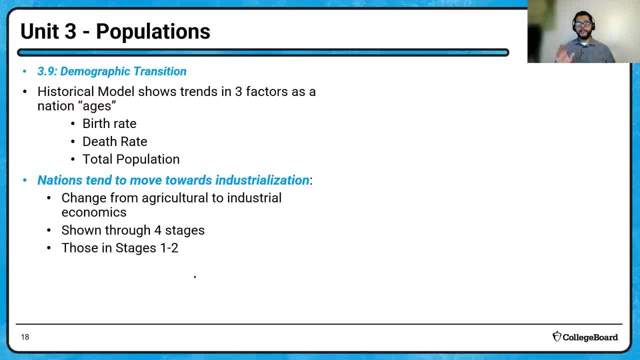 very few, if any, are in stage one anymore, right, so stage two is probably where we began for most. and those younger nations. they tend to have younger populations, um, and unfortunately they have a higher infant mortality, and one of the reasons why they have such a high number of 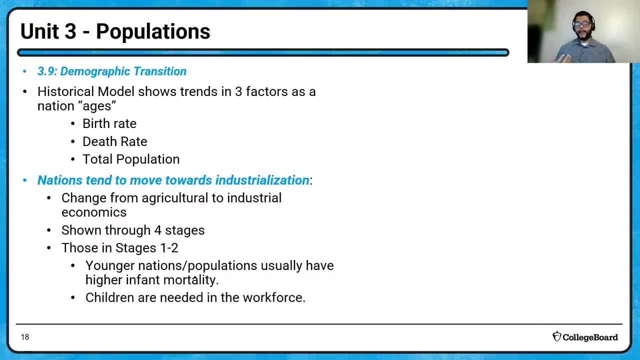 children is that children in the workforce tend to be a um, they tend to be an asset right, and so this is where we end up relating back to our population pyramids. okay, so this is an example of an important thing to think about, because a nation in stage one or stage two would likely be 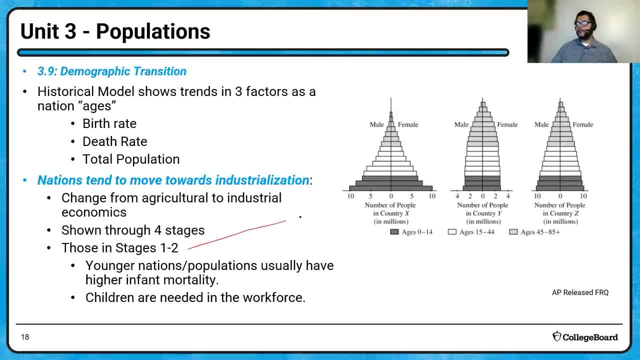 right over here, okay. so stage one, stage two: they're going to be looking at that pyramid, okay, whereas a nation in stage three would likely be over here- sorry about that- and a nation in stage four would likely be in this one, okay, off to the side. so that's an important factor to think about, um, and we're going to show you. 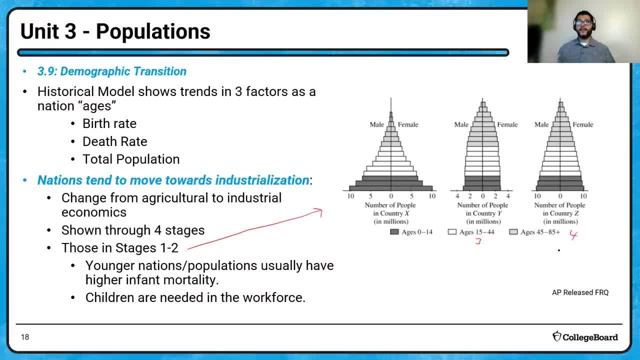 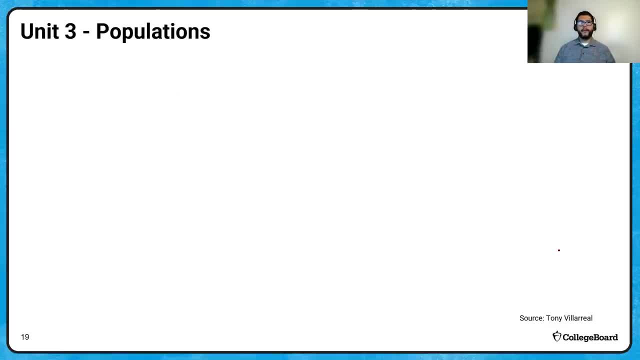 this and this is how the demographic transition is tends to be represented to us. so important to note that that's something you'll definitely see on a question. and then here, here's what it looks like. so, um, this is my kind of rendering of what this would look like. so if 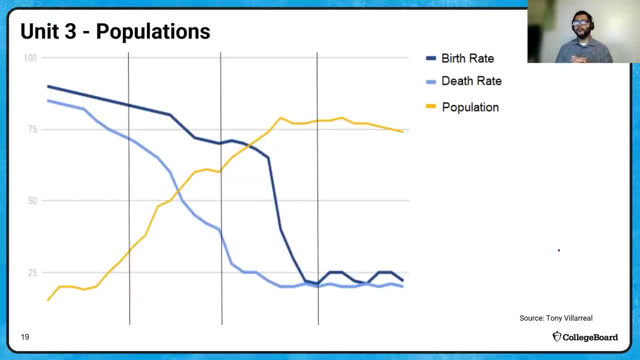 we look at it, the dark blue line is our birth rate, the lighter blue line is our death rate and our yellow line is our population. so, again, this is not a specific country. this is just the general view of demographic transition, right, and so what tends to occur here is phase one. you end up having 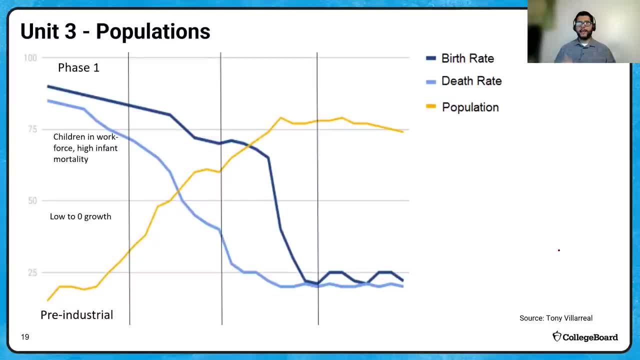 a higher number of children in the workforce, mortality is up, and then they tend to have zero or low growth. right, this tends to be because, in fact, they are going uh, to have a much higher infant mortality rate. health care is not as widely accessed and it takes a while. 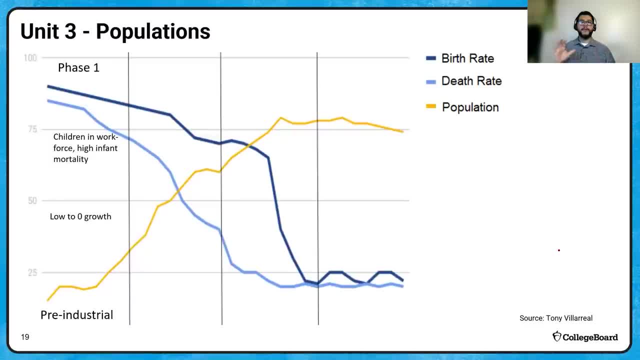 so again, very few, if any countries are in phase one to be some indigenous populations, but even then, that's um. i highly doubt that there's anybody left now in phase two. this is where medicine is improving. this is more of a developed nation. sanitation is improved and food production is becoming improved. what that does is it leads to. 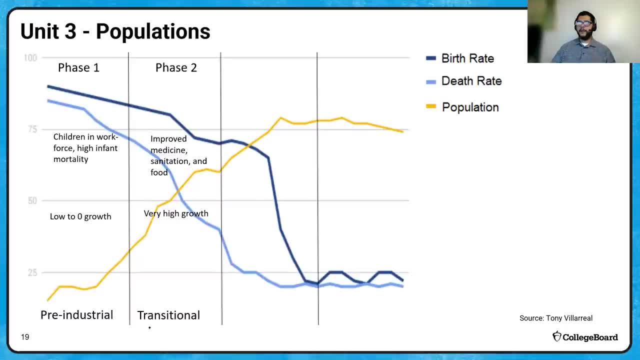 a very high growth rate. so you see, right here, if you think about it, if we were to separate this line right there and this line right there, that's kind of like a j curve. that's the fastest point of growth. right, the population is going up and up and up. and then what's happening to the birth and 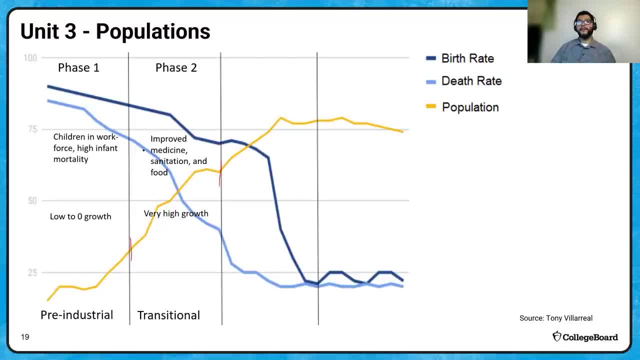 the death rate it begins to drop. it's still high, right, but the death rate tends to drop much faster, okay, and because of that the population number is able to grow bigger. so because the gap between the two lines here, between the blue and the, the dark blue and the light blue, gets bigger and bigger. 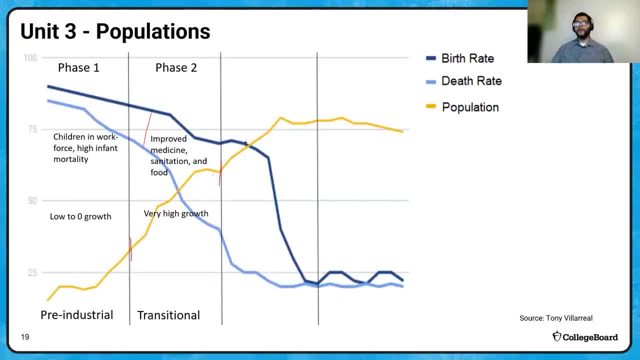 then the population can grow faster and faster. and then what we see in stage three: that's where we start to get higher education. we mentioned this earlier. right, the education improves for women and for men. but because the education is higher, the health care has gotten better. there tends to be a much lower mortality rate for infants, and that leads to much slower. 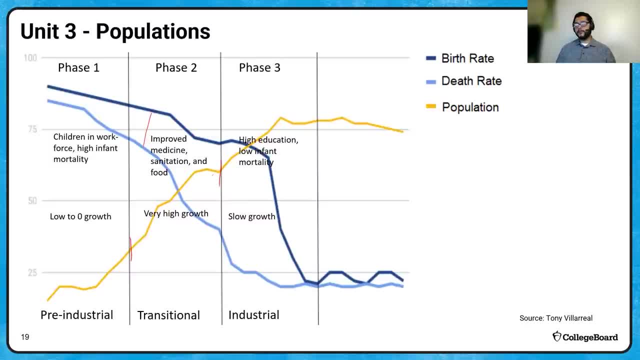 growth. so they're still growing, but it's become to a point where the gap is shortening. so over here, remember, the gap was getting bigger and bigger, and now the gap is getting smaller. okay, and then finally, when you get to phase four, this is where the population has very high education. 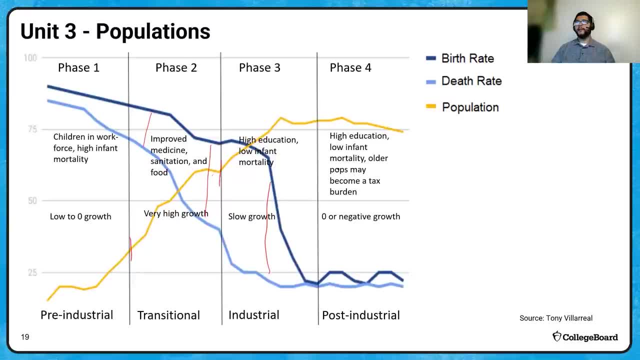 the infant mortality has remained much lower, okay, and the older populations become somewhat of a tax burden, right, um, and so because of that, you end up with zero or beginnings of negative growth, okay, and then down here, take a look at our birth and our death rate. they're now meeting up again, but they're much lower. so up here they were very close. 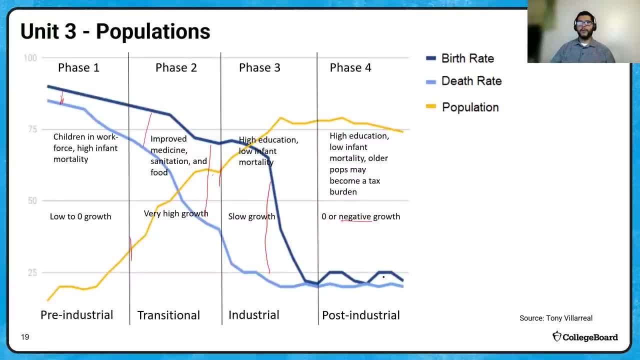 to the birth rate. but now they're down here and they're very close again, but look at how much lower they are. and then with our population this is now stabilized and that's more of that carrying capacity line and it may even begin to decline. and of course, if you're in human geo and you've 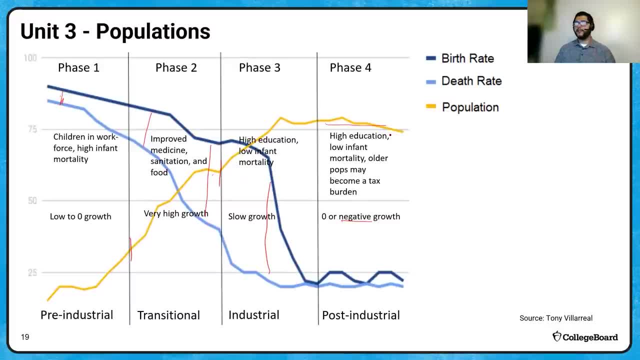 taken that you'll see in phase five. there is a clear decline in those and you do see that in some countries. so that's another point i do want to make a note of. they will ask you examples sometimes of what country is an exemplary of phase three right? 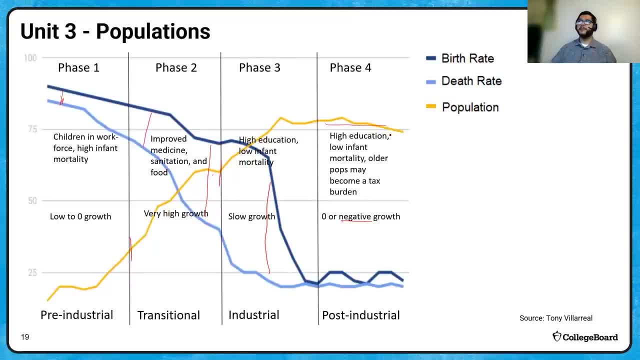 So for now, United States tends to be a phase three nation right, Whereas Japan or parts of Europe tends to be in a phase four. They're much stable, they're older populations and they're not growing anymore, And then phase two would be something like China or India, which is 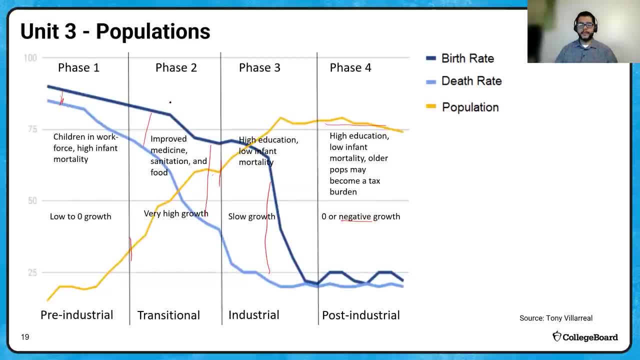 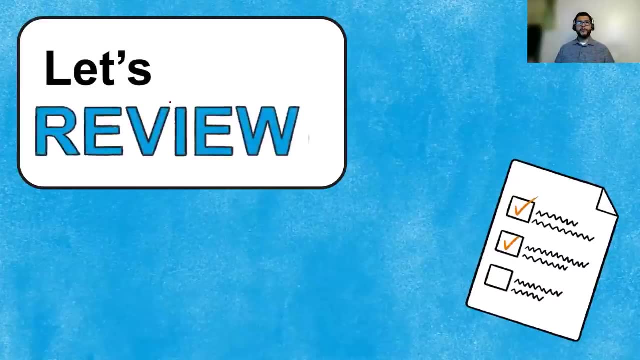 very rapidly growing. right now, India is actually surpassed to be the biggest group, the biggest population. in the next 10 or 15 years they're going to surpass China. So, okay, So that's a lot of information for unit three. So let's review and do some practice. 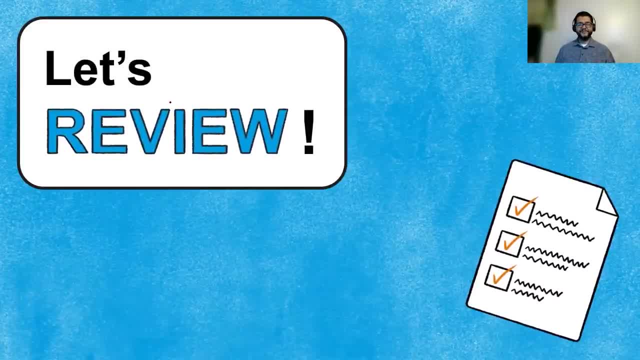 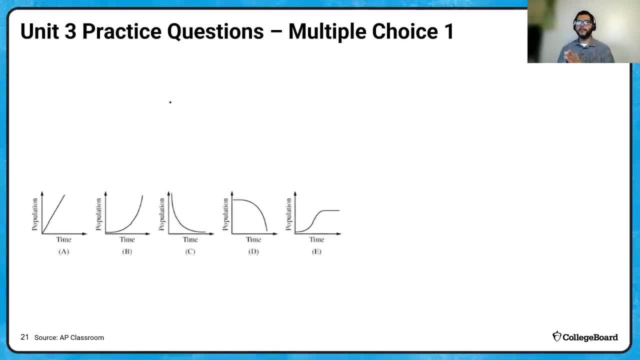 right, See what we know, or what we think we know right. So let's take a look. So here's first multiple choice question example. And if we look at these we have graphs, So we have population and time And again always look at the graphs first and say, all right. 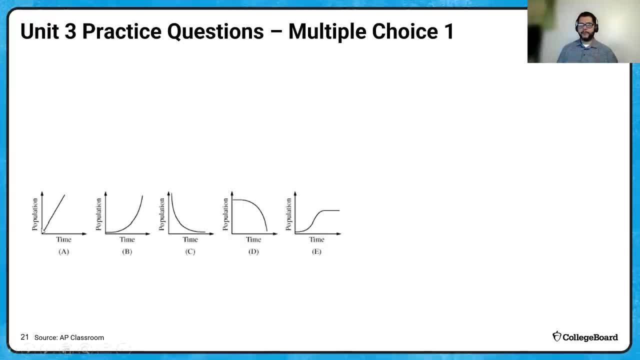 what is happening. So in A I see a movement up. right In B I see movement up, but I see it more slowly and then faster and then slow again, And then I see over here in C that it's more of a. 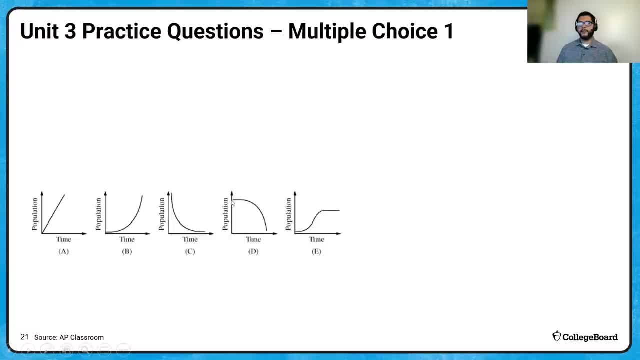 decline. it's more of a drop over time. And then here the population kind of goes, starts off stable and then drops, And then we have a population that starts off slow, speeds up and then slows down and again right. So let's look at the question: Which graph best illustrates a population that was growing? 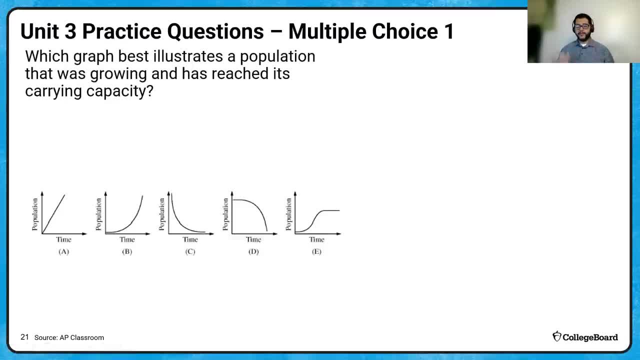 and has reached its carrying capacity. So this is why I ask you guys to make sure you look at the choices first, and look at the diagrams and read what you have to read And from there you can make your decision And, honestly, if you did, you take a look at this. 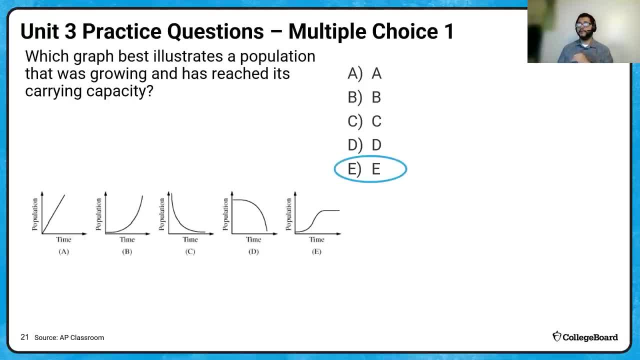 the answer should be pretty obvious that it's letter E. Right, They've reached that carrying capacity And again, it's not a perfect world where they all get a memo and they stop reproducing and the population stabilizes. But that's the exemplar that they are showing here right Now. this might be considered a 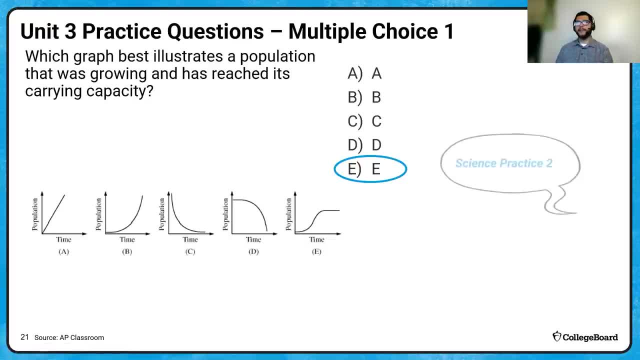 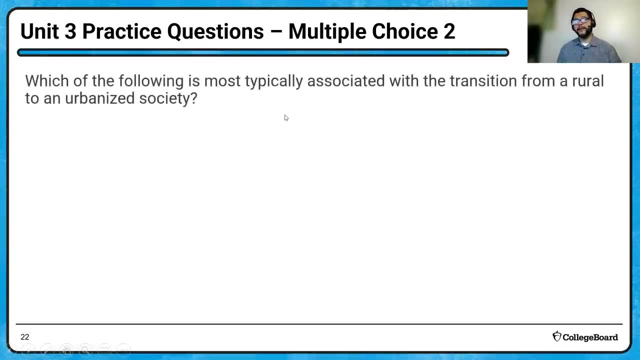 skill number five, but there was no data analysis. So this is actually a practice two, right, And if you want to know a little bit more about carrying capacity, you can look back at topic 3.4,. okay, So question two: which of the following is most typically associated with the transition from a? 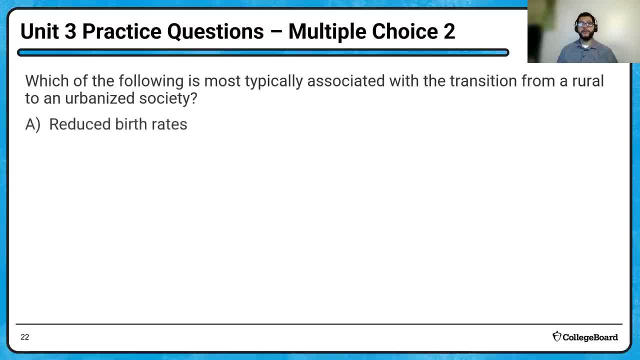 rural to an urbanized society. So is that going to be a reduced birth rate, a reduced need for sewage treatment facilities, increased rates of population growth or an increase in air quality in urban areas? So if you think about this right, this is a basic concept type question. 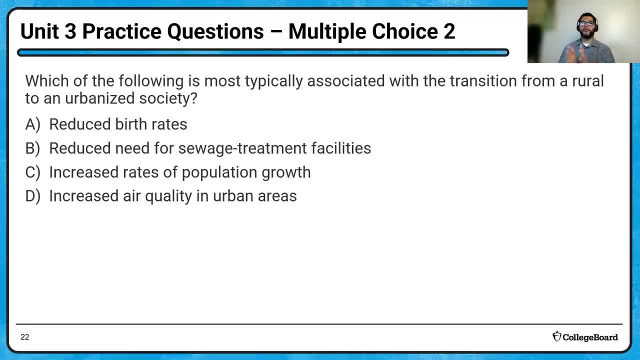 And they're asking us: you know what's going to happen when we go from rural to urban? Well, if we think back to demographic transition, we should remember that you're going to end up with lower birth rates, okay, So this is going to be one of those. do you know the concepts? That's? 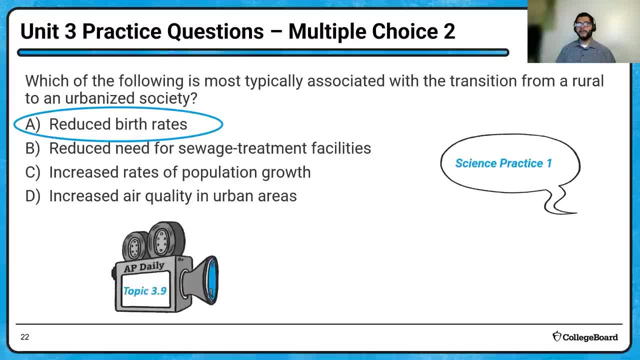 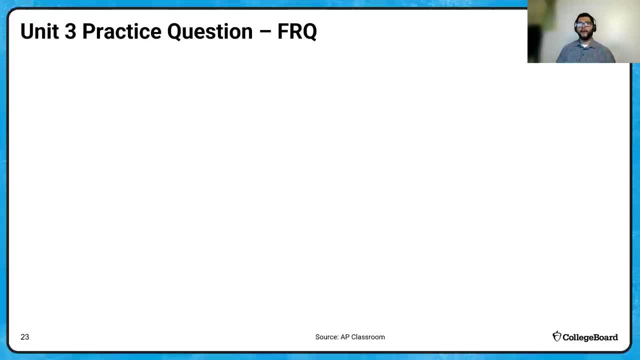 a practice one type question, okay, And if you need to review that, you can check your AP daily videos out. And now we're going to look at a free response question, So let's take a look at that one specifically. So this is a big one, right? So I recommend, once we go through all these sections, 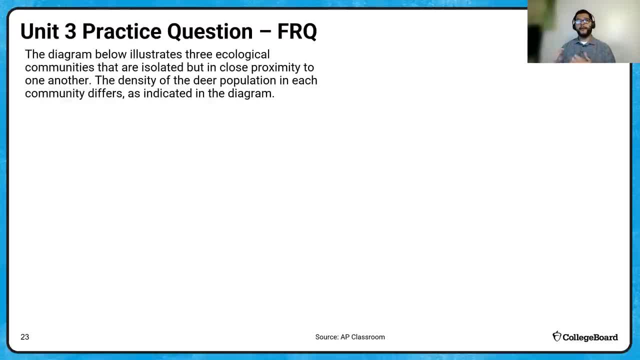 if you would like to pause the video and read it more in depth and kind of write your own answers out before we get to the end of the session, you can do that. So if you would like to pause the answers, that'd be perfect. That way you can see all that and not spoil the ending so much. 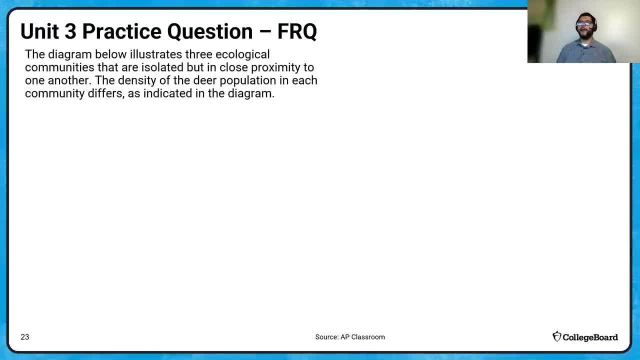 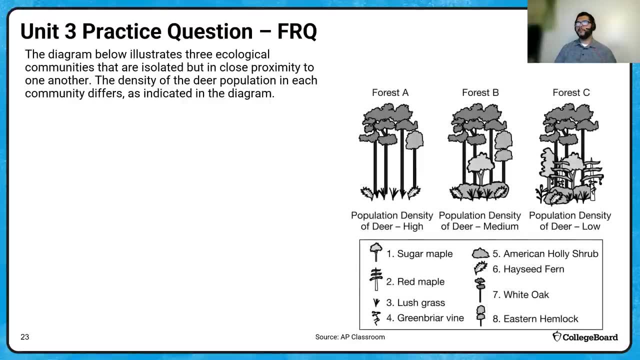 right. So here we're talking about deer populations And they all show us three ecological communities in close proximity And that the deer population differs as indicated in the diagram. So if you look right here, high deer population, medium, low and then the 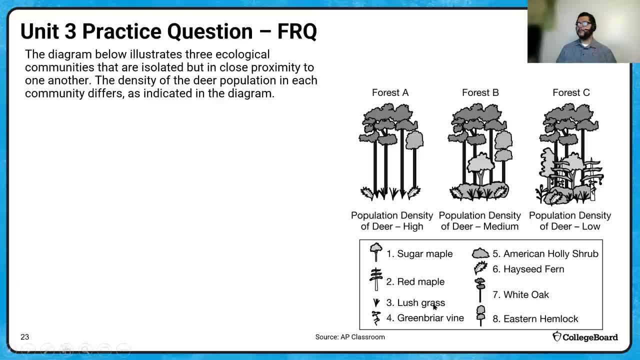 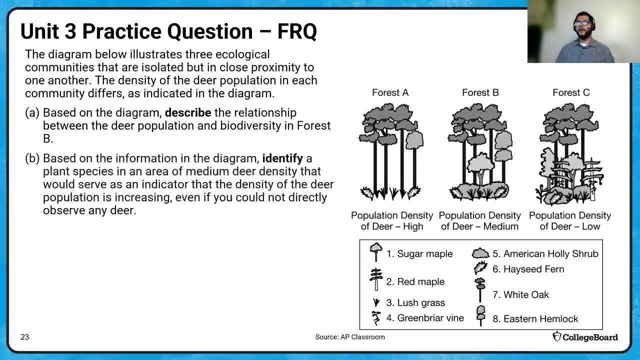 different species of trees. right, The different maples, grass, vines, shrubs, ferns, and oaks and hemlocks. Okay, So describe the relationship between the deer population and biodiversity in forest B. Okay, so that's our medium population Here. identify a plant species in an area of: 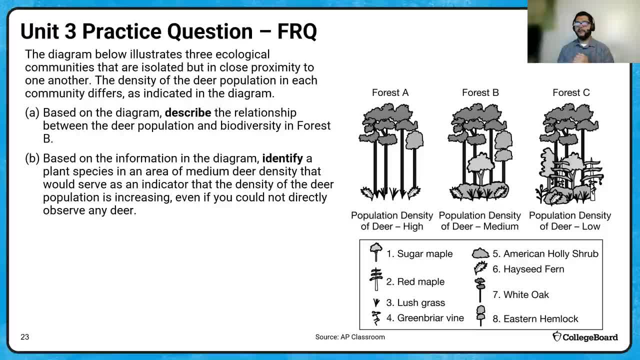 medium deer density, that would serve as an indicator for the density of that deer, even if you couldn't directly observe the deer. If there are no predators of deer, explain why the density of deer population will reach a level where it will not increase further. 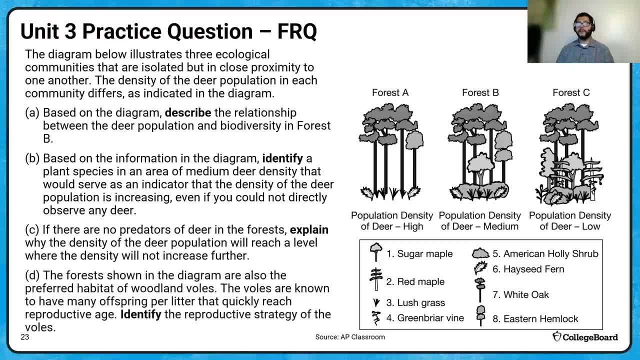 And then letter D here is asking us to identify the reproductive strategy for the voles that are known to have many offspring per litter that quickly reach your productive age. Okay, so if you want to pause that and try to write some answers down, that'd be great. 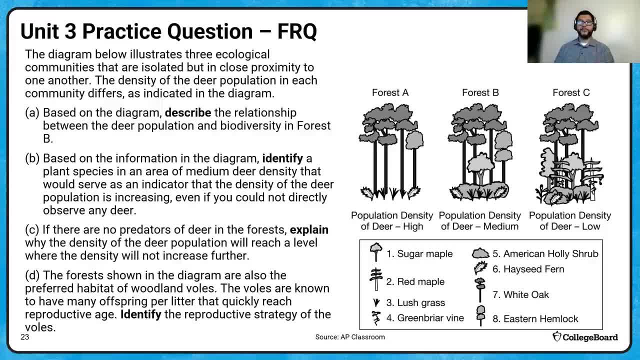 If not, here's the rest, because our FRQs are long questions. Remember that is something you do have to build stamina for. So if you haven't been practicing free response questions, definitely something I would recommend you continue or start to do right away. 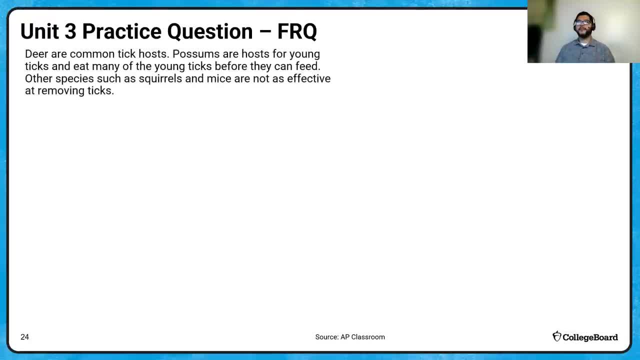 Okay, so let's look at the rest. Deer are common tick hosts. Possums are hosts for young ticks and may eat many of the young ticks they can feed. Other species, such as squirrels and mice, are not as effective at removing those. A local homeowner proposed improving the squirrel habitat to reduce. 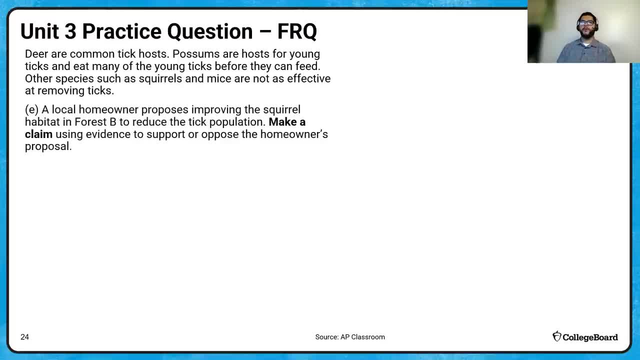 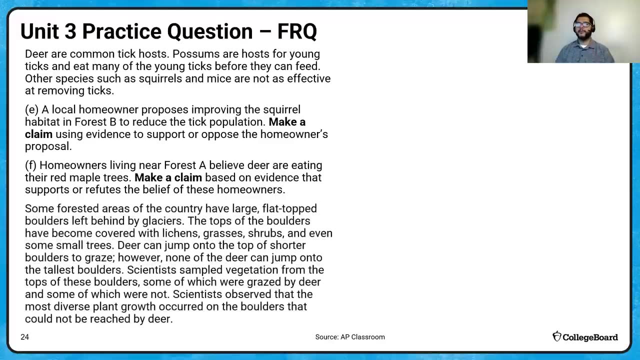 tick populations. Make a claim using evidence to support or oppose the homeowner's proposal. Homeowners living in forest A believe deer are eating their red maple trees Make a claim based on evidence that supports or refutes the belief of those homeowners. And then here's some more information: Deer can jump to the top of shorter boulders. They can. 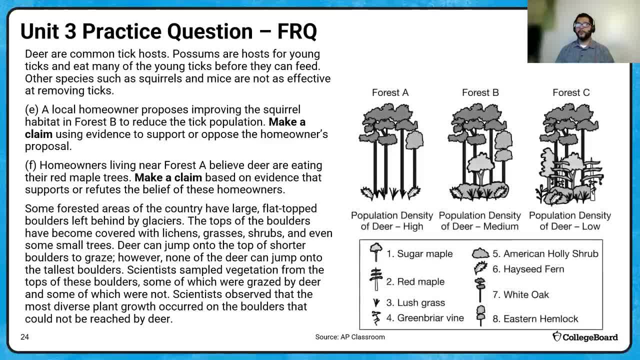 graze. Scientists sample vegetation from the tops of these boulders, which were grazed by deer, and some which were not. Scientists observe the most diverse plant growth occurred on the boulders that could not be reached by the deer. So make sure you read that and look at our graphs And if you, 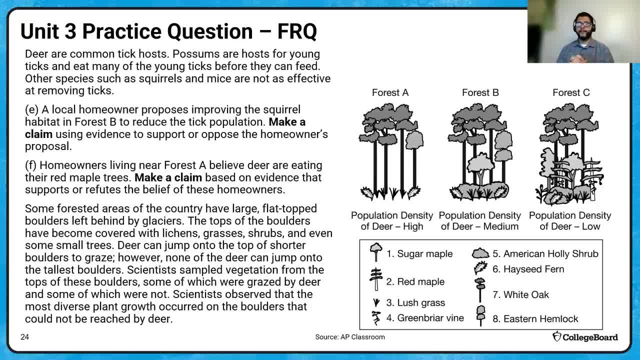 want to pause and answer these questions, please do, And then make a note here that you see here these are make a claim questions, So you're going to see the back half of this question and the next few sections. it's going to be more of an experimental design. You can tell it's a. 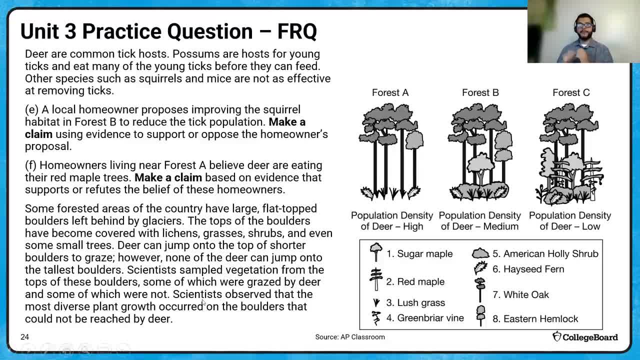 giveaway because they're talking about scientists. When they start talking about scientists, you know there's going to be a question about independent variables, dependent variables, hypotheses, what are changes you could make? So, but the first part is very, very generic. 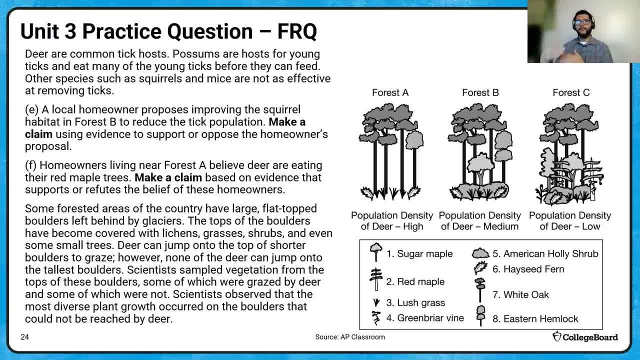 AP environmental questions, where it's here's a problem, make a claim or propose a solution. So when you see those terms, that means you're going to have to pick a side and you're going to say something. So be prepared to do that on those, Okay, And then identify the independent. 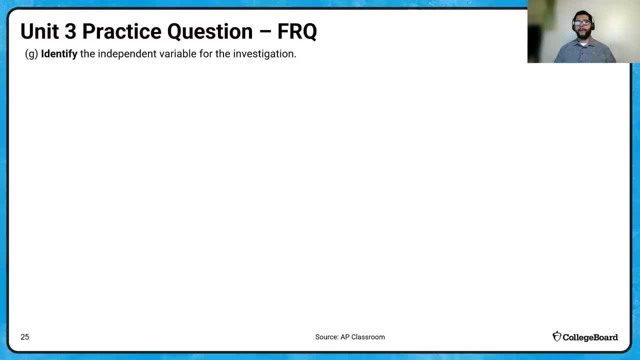 variable for the investigation. There you go, There's our, our giveaway: Identify a modification that can be made on the results of their experiment and how it alters those results, And then describe the steps that lead to the establishment of a forest, once soil formed in that study area. So this is going to be a little bit of a mix. 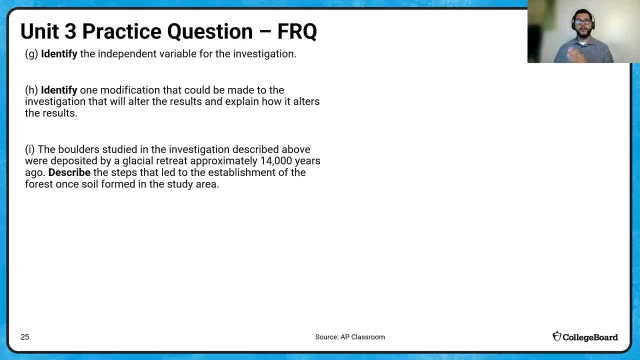 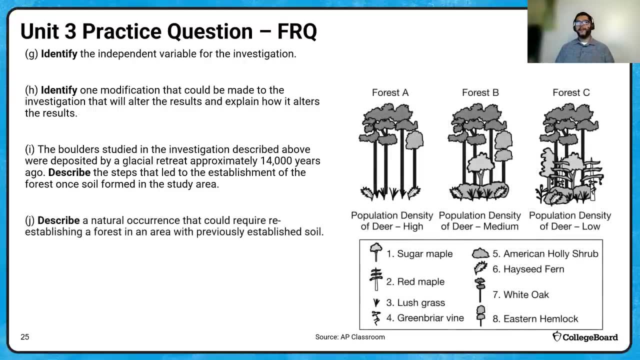 As you can see, there's never a question that has just one unit to it. It's got many different units And we'll talk about that in a little bit, So let's go ahead and do that, Let's talk about that in the end, And then the last portion here describe a natural occurrence. 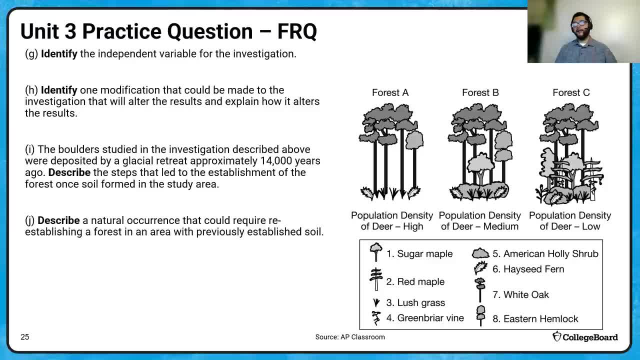 that would require reestablishing a forest in an area with previously established soil. So you see, there's some unit two in here that you're going to see kind of ties in. So if you'd like to go ahead and pause the video and answer these last portions of questions and then we're going to go. 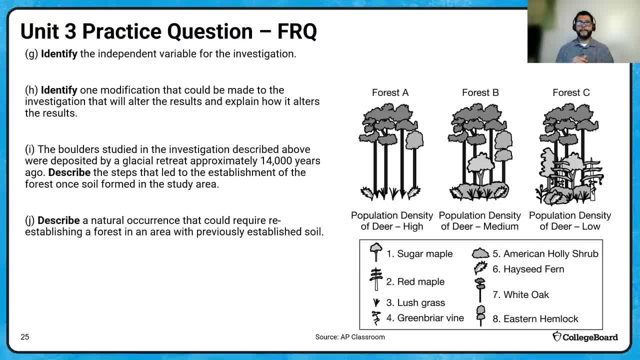 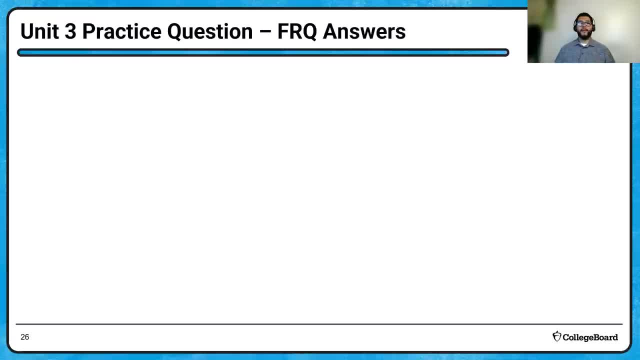 over the answers in the next slide. Okay, Hopefully you did that. If not, that's okay, Let's just go to the answers, right? So part A: the question was for you to identify a to describe the relationship, excuse me, between deer population and biodiversity in B, And you'd have to say that. 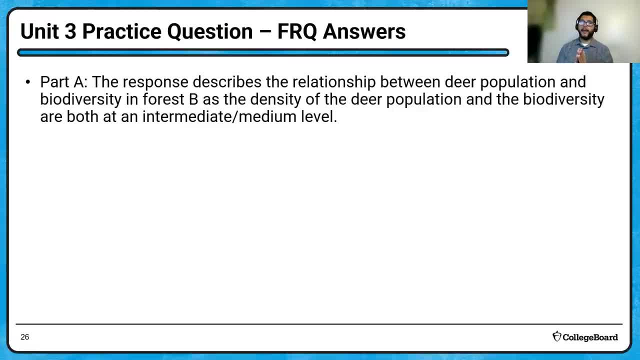 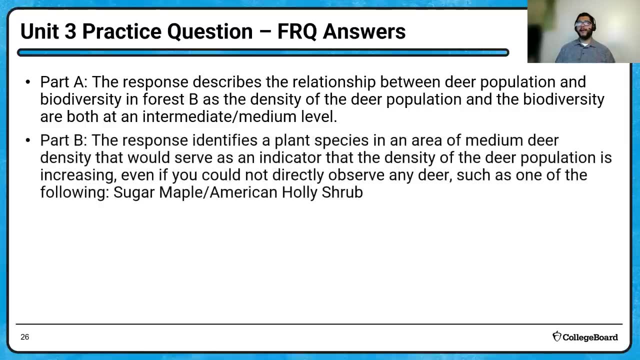 the population. the density of deer population and biodiversity are at an intermediate and medium level. So you'd have to notice the tree species, maybe count them and compare them to groups, to forest A and forest B. Part B says to identify the plant species of medium deer density. That's going to be an indicator if they were there. So if you, 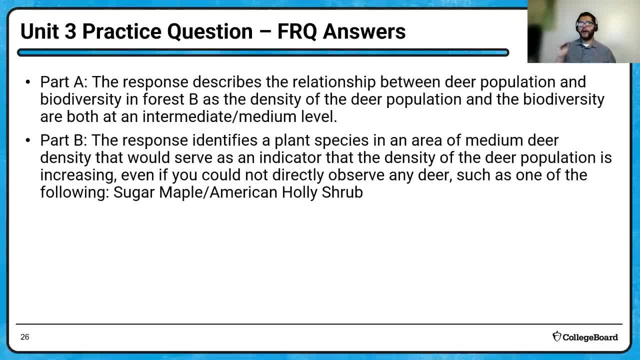 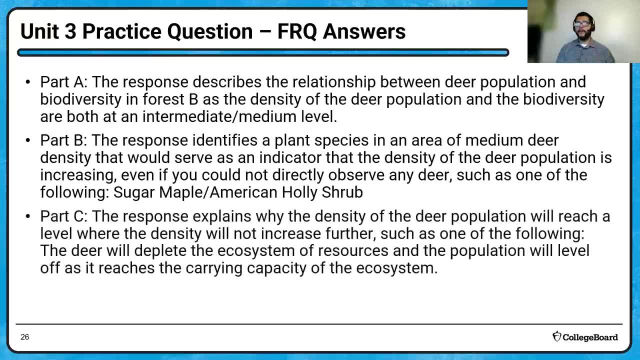 couldn't directly observe deer. you could say that the sugar maple or the holly shrub was in different number than usual. So that's something you'd want to consider there In part C. you'd have to explain why the density of deer is going to reach that level. 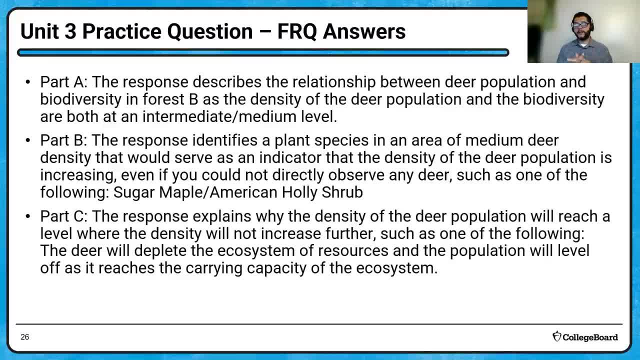 when it won't increase. So that would be something where you talk about carrying capacity and how it reaches that carrying capacity due to a resource of some sort, right? So there's population portion there And then part D. here the response identifies the reproductive strategies. 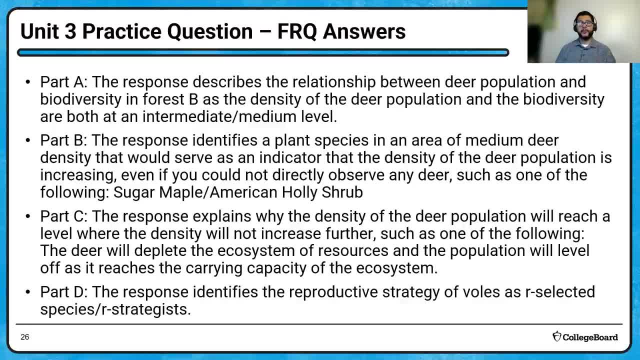 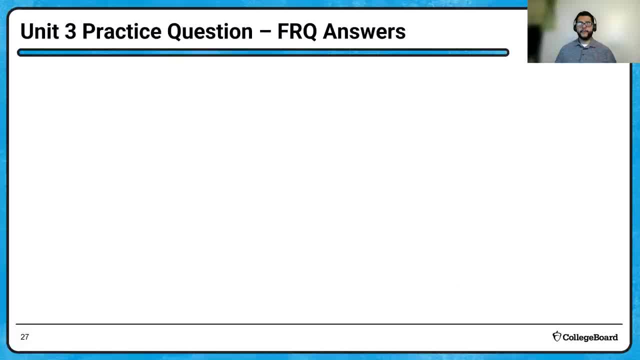 as are selected because they're having lots of babies with little parental care. So you see, here it's mixed in And then we're going to see in the next portions. here's our experimental design part. So the claimant evidence is going to be well. the homeowner's proposal should be opposed. 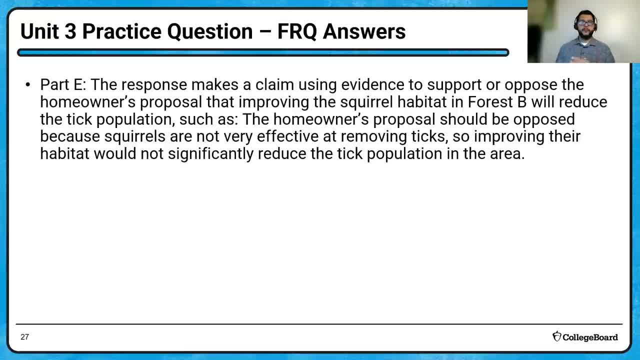 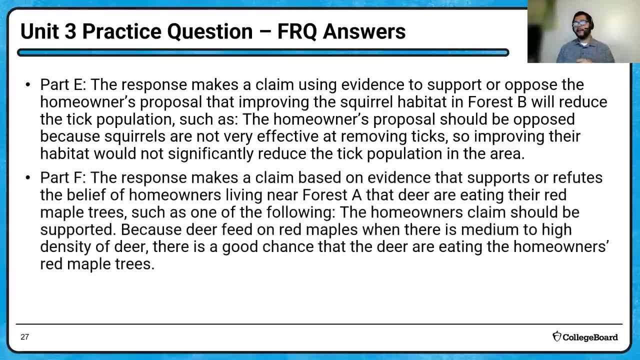 because, as the paragraph explained, squirrels are not effective at removing those ticks, So that wouldn't be a very good strategy. Part F in this one we'd say that we could either support or refute their claim and that forest A have deer eating their red maple trees, where you could say: 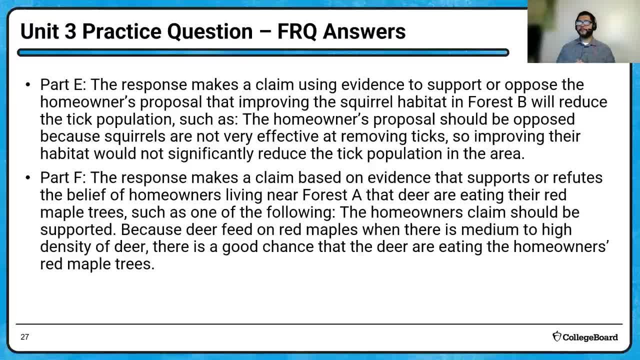 that it's supported because, as the deer feed on those red maples, there's a medium, higher density, medium or high density, and that's going to end up bringing down the red maple population And then part G is going to be where you. 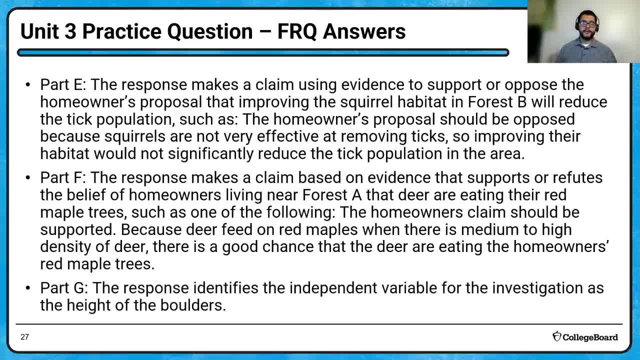 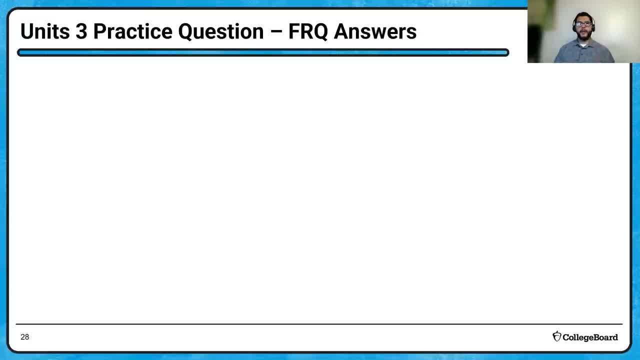 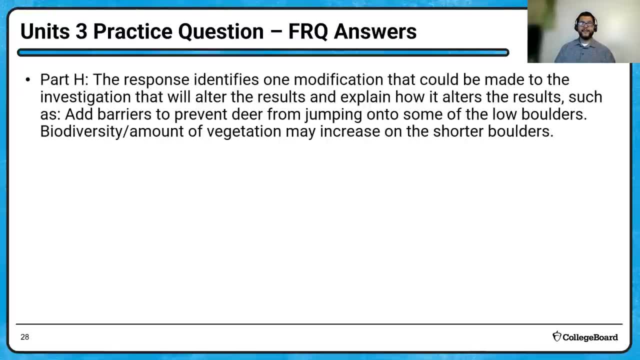 you identify the independent variable as the height of the boulders, because that is going to be what changed and what the populations look like on the bottom and the top, And then part H, right as we go halfway through the alphabet. we have that, the response telling us that you could. 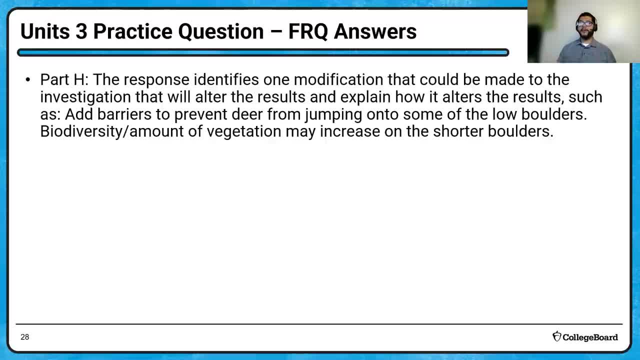 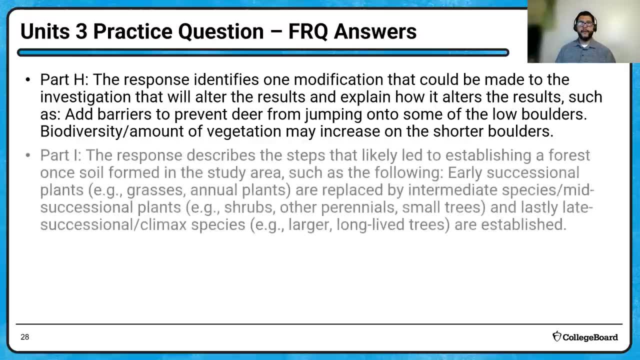 find ways to alter the results So you could add barriers to prevent them from jumping to the low boulders and see if that increases the population and vegetation on those. And then part I is going to be where you can, you know, look at the study and say: well, these early successional plants are 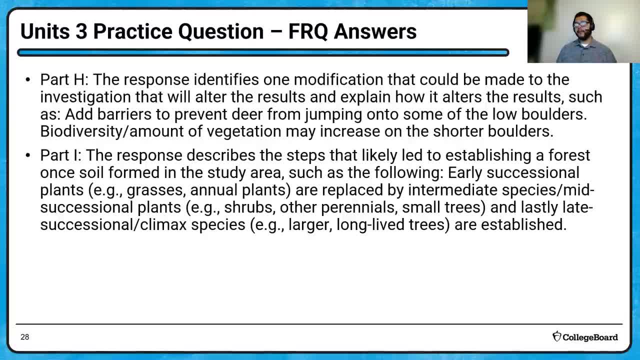 going to be replaced by intermediates. And then, lastly, the climax community. So this is asking a succession in here. So make sure that we're familiar with those And if you need some refresher on succession, that was a video two topic or you can go to AP Daily. And then, of course, 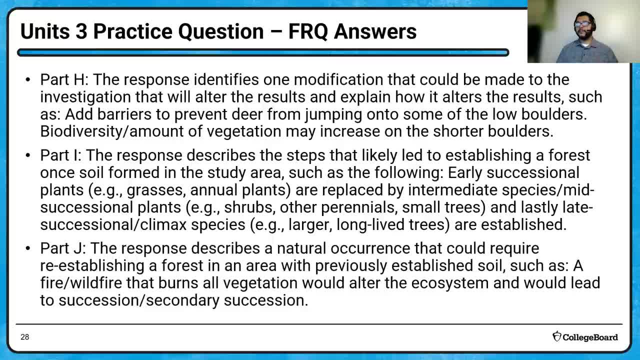 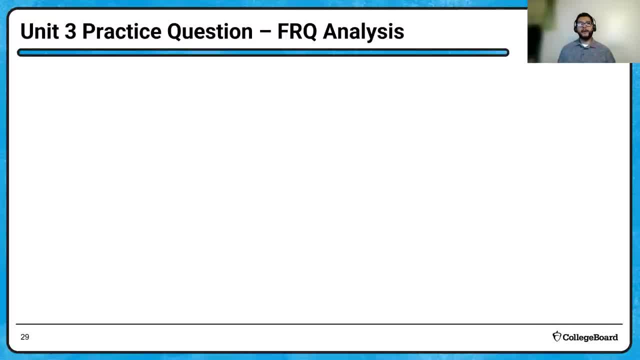 this is going to be where there was previously established soil, We would have to say that that would lead to secondary succession. Okay, And so if we take a look at that, we want to ask ourselves, right, what did we look at in this FRQ? Well, we look at the FRQ and we see that. 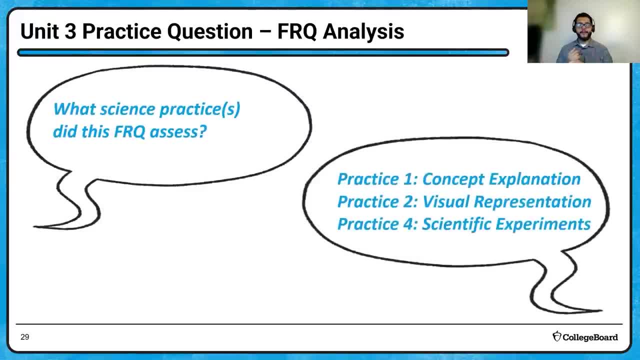 there's several practices we looked at Now. they had a concept in there where they were asking us about succession. They were asking us about the different. what is this showing? or how do we know this problem exists And there were definitely visuals because they showed us those population. 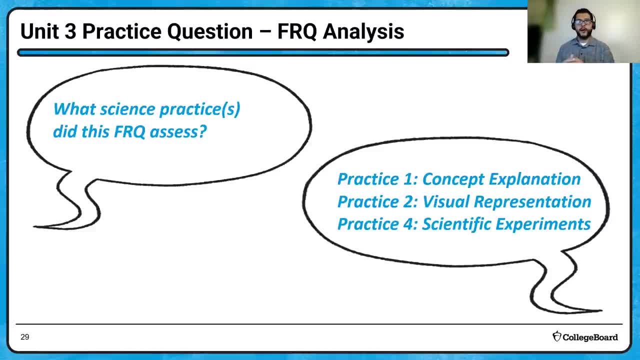 in the forest. And then of course we saw our scientific experiments where they were asking about independent variable. How do we change the experiment, That kind of stuff. And then again I do want to show you here that when it comes to the topics, not one unit or topic is going to be. 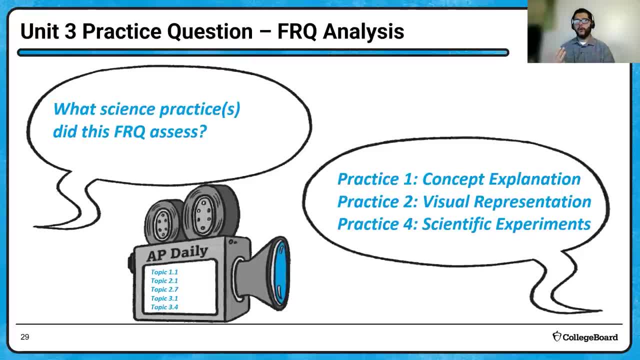 asked in an FRQ. It's going to be multiple, So we had some 1.1,, some 2.1, and, of course, some of the unit three as well. So be prepared for that, because it's going to be all over, All right. Now. what should we take away from all of this? 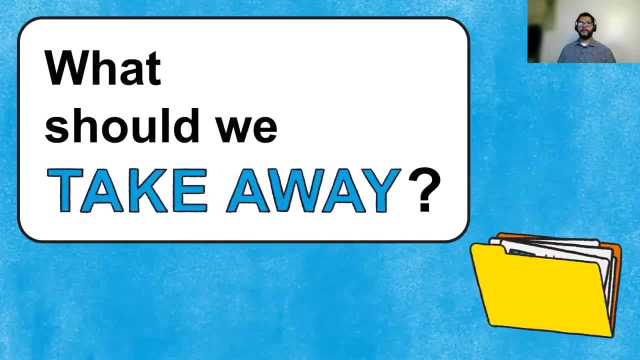 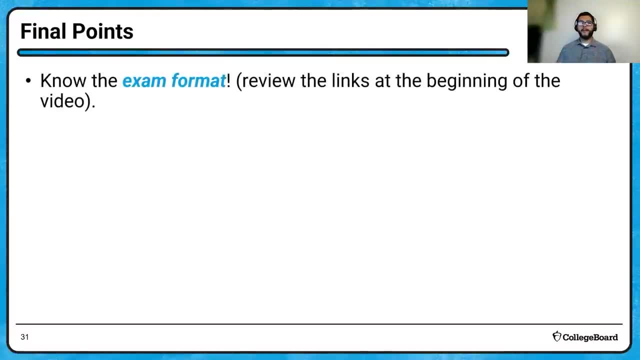 right, That was a lot of information. Let's see what we know. Some final points. Again, make sure you're familiar with the exam format. If you need help with those, you can review the links at the beginning of the video or you can go back and look at video one and video two to help. 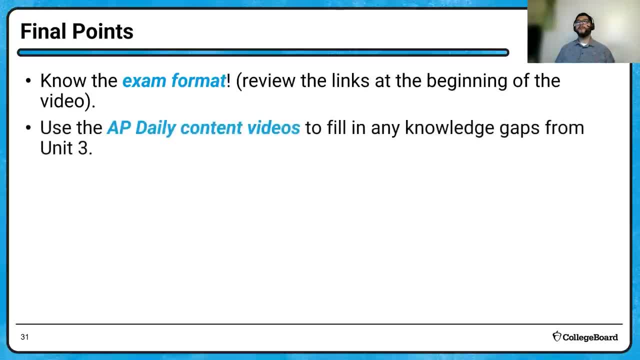 you refresh on some of those. And then, of course, please review the AP daily content videos to fill in those knowledge gaps. right, If there's something from unit three, like there's some numbers that we didn't get to go over. right, Like the human population. 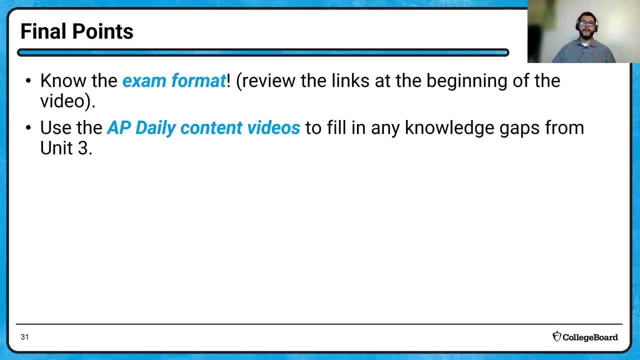 or the population of the US. those are going to be big ones And if you need more math practice, you know. please make sure you check those AP daily videos on AP classroom And then be prepared to go a little more in depth. So, while we just scratched the surface today, make sure to. 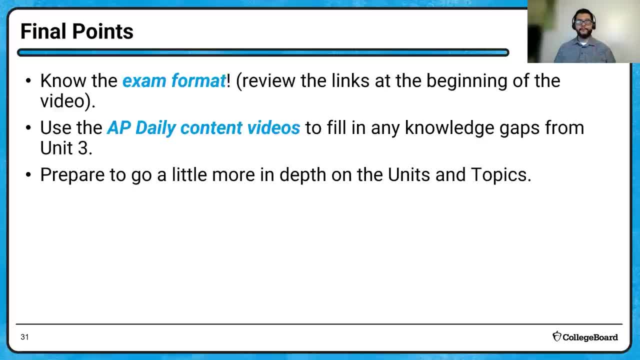 understand you're going to have to go back and know this stuff pretty well And then, of course, be prepared to use math and be comfortable. I'm going to go with practice four And this is. you know, if I had to characterize unit three with 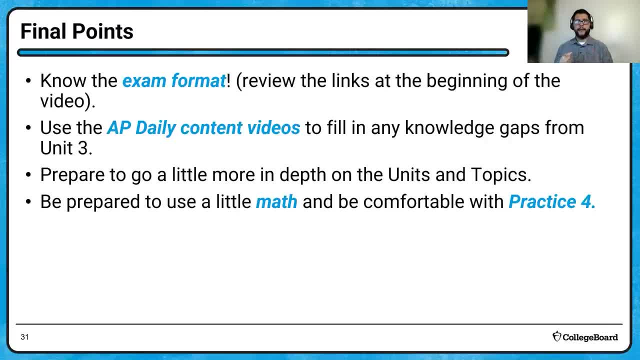 two words, I would say graphs and math. right, If you can identify all those graphs, all those charts we're talking about, then you should be good. And then, of course, be comfortable with those biological populations and human population questions, so that you know the difference and you 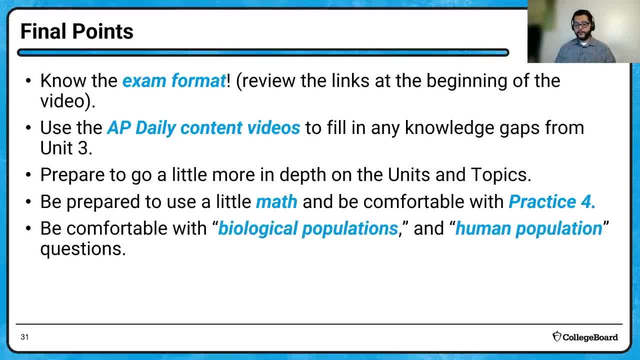 know what they're asking. You know, because you can't really propose tax policies to help. you know, endangered species population go up. I mean you probably could, but it'd be a difficult sell right, Especially depending on what the question is asking. Okay, so if you'd like to do, 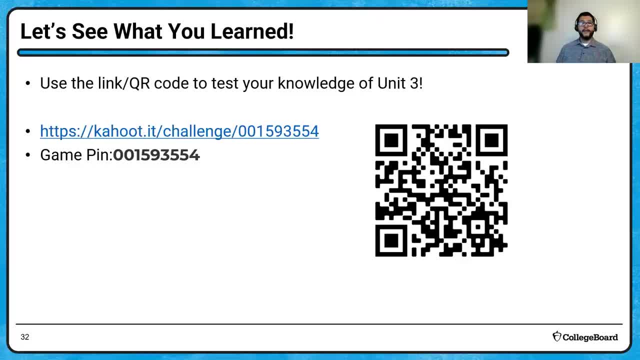 some practice and see if you learned what you know what you learned, then please by all means take a chance and scan that and you can go to that Kahoot with that game pin And you can practice on your own. So that's open to anybody who's watching the video And you can do some practice. 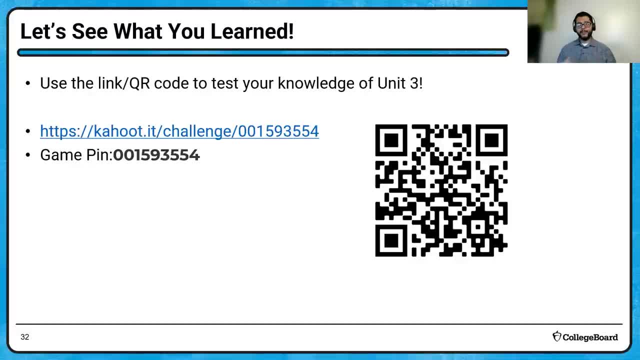 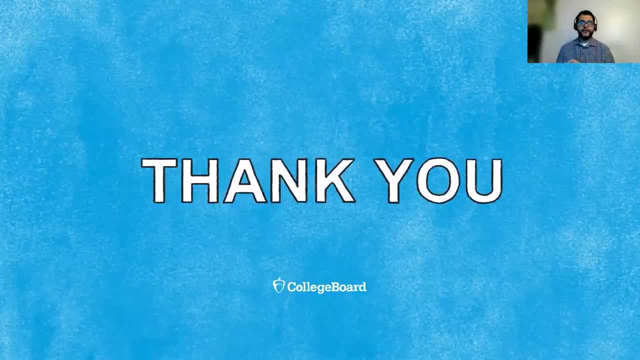 questions. So hopefully this was helpful, guys. I really hope that you got what you needed And I want to say thank you again for watching And just a quick shout out to my students at SA3.. Keep on studying. And to my own kids, Anthony, Annie.